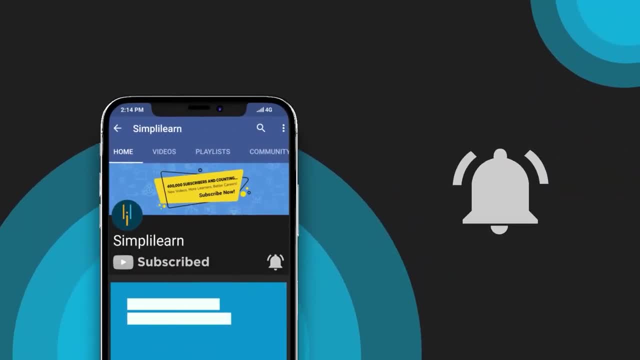 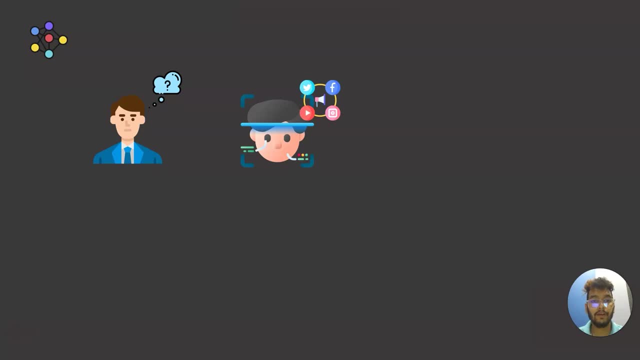 Have you ever wondered how facial recognition works on social media Or how object detection helps in building self-driving cars? It is all possible thanks to Convolutional Neural Networks. Hello everyone, I am Mayank and welcome to Simply Learn. Today we will. 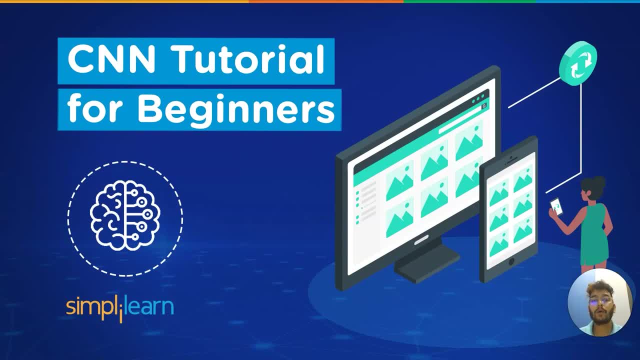 take you through a hands-on lab demo of how we can use CNN model for image classification in machine learning. For amazing videos like this, subscribe to our YouTube channel and press that bell icon to stay updated. In today's session, we will discuss what CNN model is. 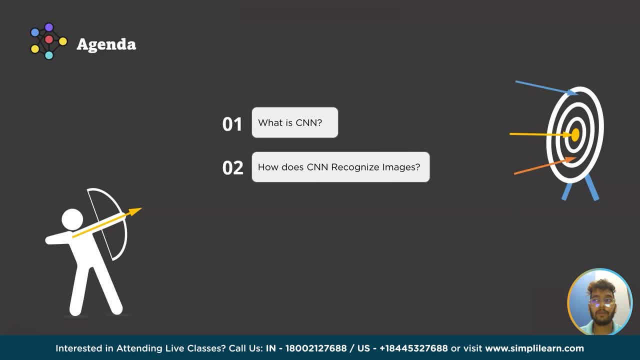 and moving ahead. we will discuss how does CNN recognize images. After that we will see layers in CNN. At the end we will do a hands-on lab demo of image classification using CNN. In fact, a study says there will be more than 2.3 million job openings in the field of artificial. 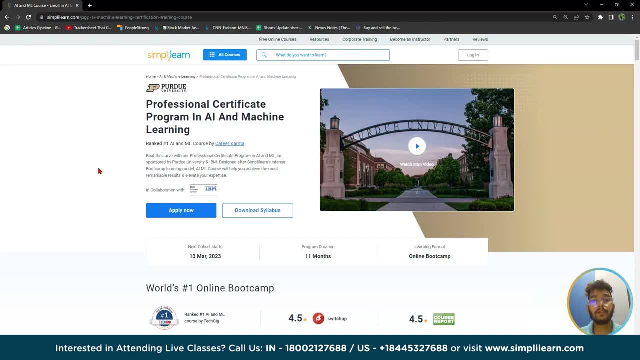 intelligence and machine learning by 2023.. But you can beat the curve with our professional certificate program in AI and machine learning, co-sponsored by Purdue University and IBM, which is designed after Simply Learn's Intense Bootcamp Learning Model AI and ML certification course. This course covers tools and techniques. 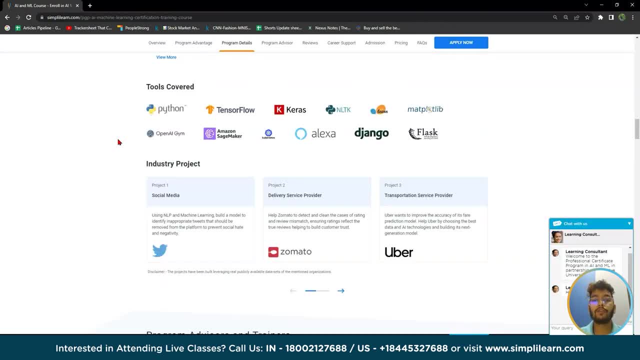 like Python, TensorFlow, Keras, NLTK and many more, along with industry projects like Social Media by Twitter, Delivery service provider by Zomato, Transportation service provided by Uber and many more amazing projects. Choosing this course, can you get hired by renowned. 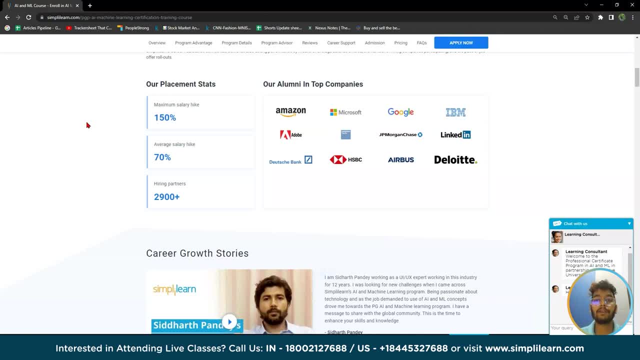 companies like Google and Microsoft. If you are interested in learning more about CNN, you can take this course, and be sure to subscribe to our YouTube channel. There are many other: Amazon, LinkedIn and Adobe- and an average salary hike of 70%. 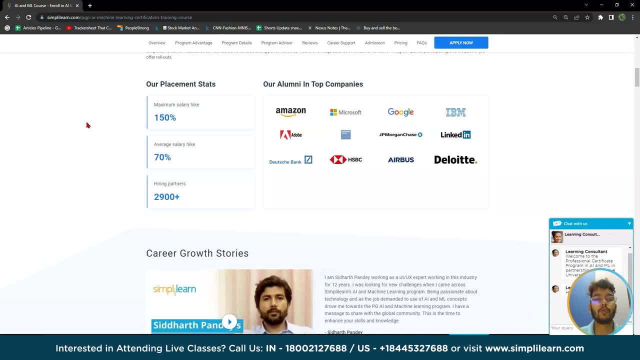 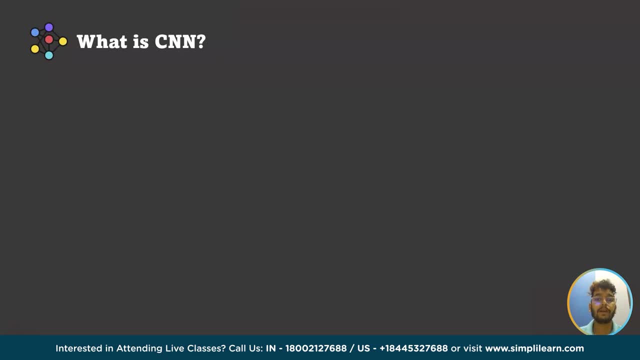 So what are you waiting for? Join the AI and ML professional certificate program and excel your career in artificial intelligence and machine learning. The link is in the description box below. Before we move on to the programming part, let's discuss what CNN is and proceed further. 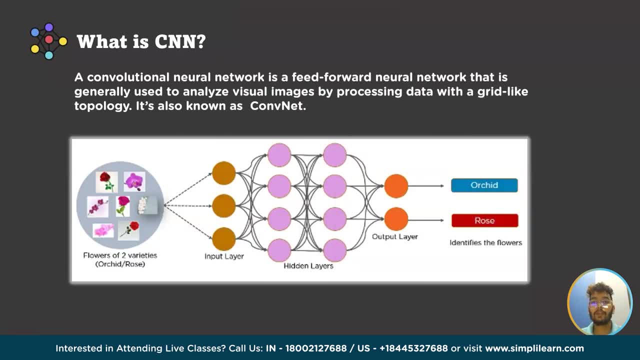 for the same. What is CNN? A convolutional neural network is a feed-forward neural network that is generally used to analyze visual images by processing data with grid-like topology. It is also known as convNet. A convolutional neural network is used to detect and classify objects in an image. 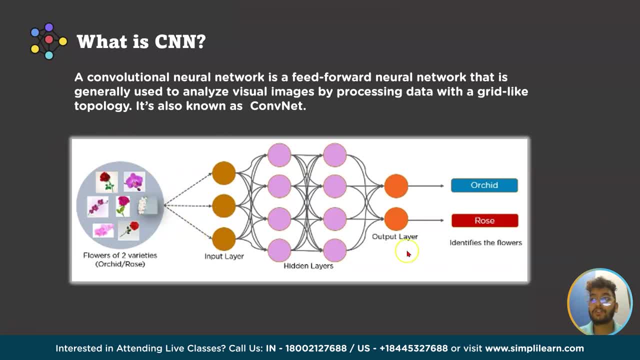 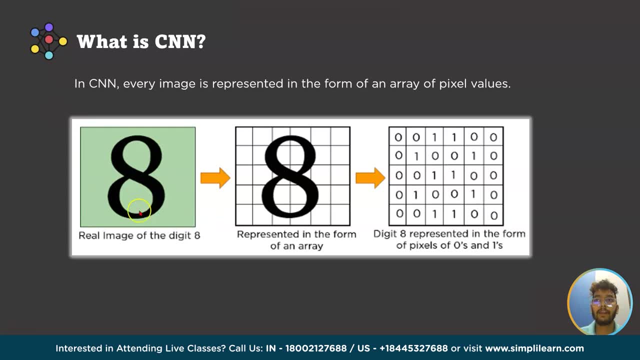 So this is a neural network that identifies two types of flowers: orchid and rose. In CNN, every image is represented in the form of an array or pixel. Here you can see, it is a real image of digit 8 and it is represented in the form of an. 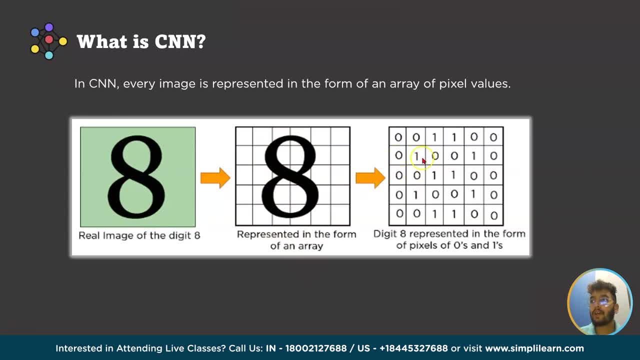 array and here 0 represents negative values and 1 represents positive values. Okay, it's creating 8 here. So digit 8 represents in the form of pixels of 0s and 1s. So now let's understand the convolutional operations using two matrices, A and B, of. 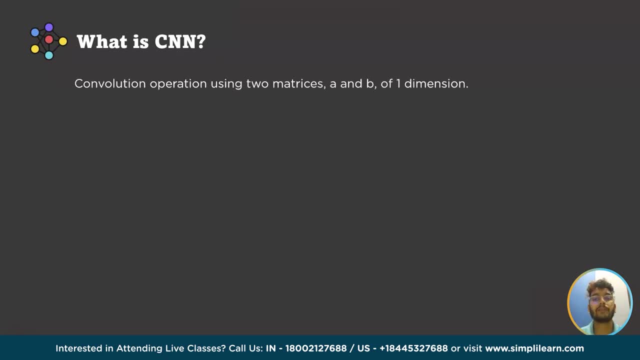 one dimension. Now let's understand the convolutional operations using two matrices, A and B, of one dimension. A equals to 5,, 3,, 2,, 5,, 9, 7.. B equals to 1,, 2,, 3.. 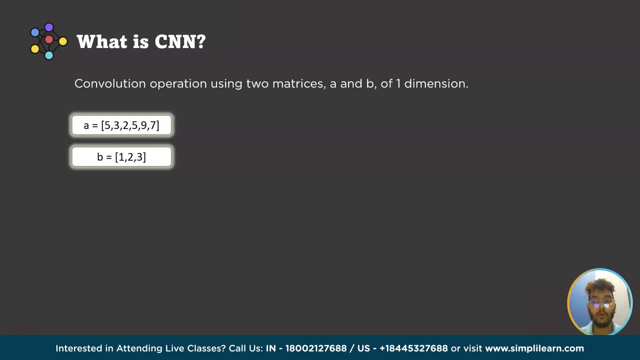 So in convolutional operations the arrays are multiplied element-wise and the product is summed to create a new array which represents A into B. So here A into B, 5,, 3,, 2, and 1,, 2,, 3, multiply the arrays element-wise and this is the sum. 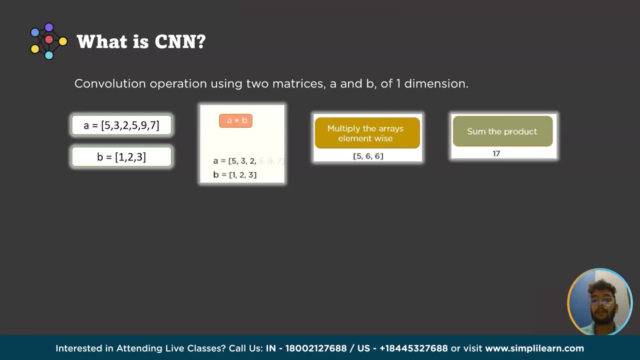 of the product. So the first three elements of the matrix A are multiplied with the elements of matrix B and the product is summed to get the result. So A into B is 17.. The next three elements from the matrix A are multiplied by the element in the matrix. 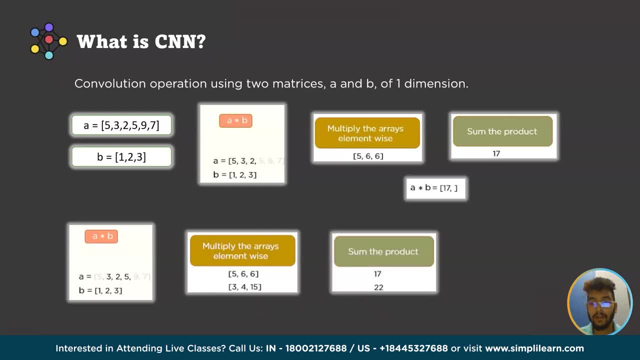 B and the product is summed up. So here, sum of the product is 22.. So A into B is 17 and 22. This process continues until the convolutional operation is complete. So moving forward. now let's discuss: how does CNN recognize images? 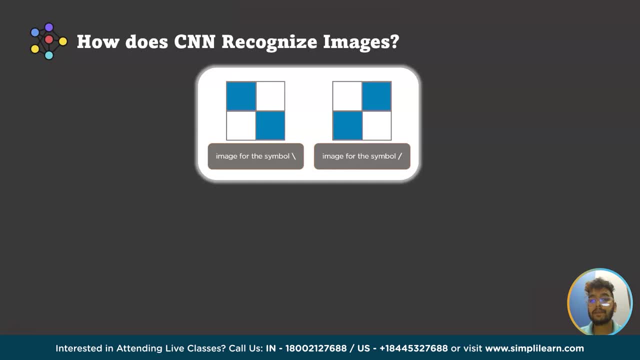 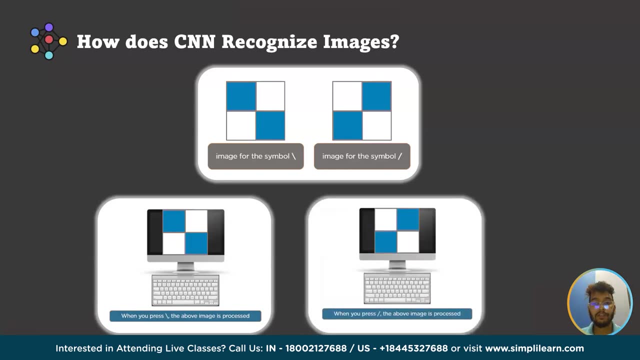 So consider following these images. The boxes that are colored represent a pixel array, The pixel value of 1 and 0. if not colored, When you press backslash, the below image gets processed, and when you press the forward slash, the below image is processed: 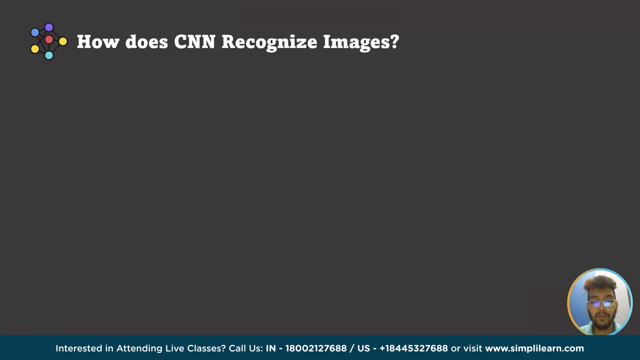 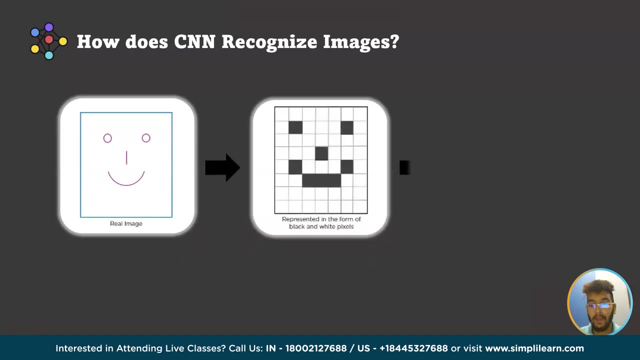 Here is another example to depict how CNN recognizes an image. So consider: this is a real image. Now it is represented in the forms of black and white pixels and this image represents in the form of matrix of number. Here you can see where. here the black part and here is one value. 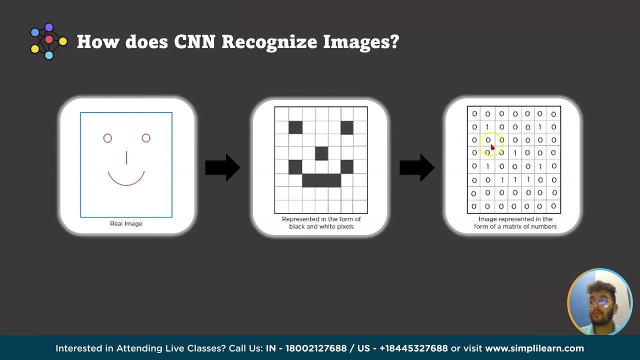 So it's creating the image, The image represented in the form of matrix of number. So, as you can see from this diagram, only those values are lit that have value of 1.. This is how the CNN recognize the images. Now, moving forward, let's see layers in convolutional neural network- CNN. 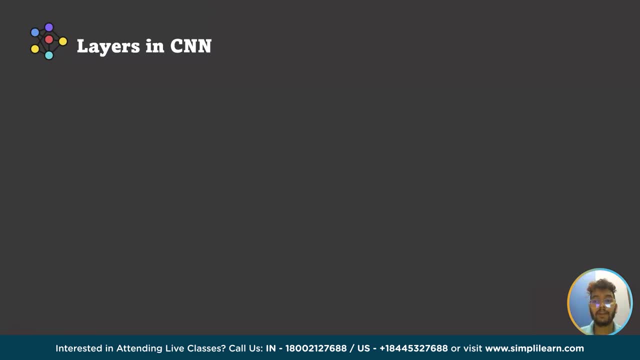 A convolutional neural network has multiple hidden layers that help in extracting information from an image. The four important layers in CNN are: first is convolutional layer, second is pooling layer, third is telu layer and fourth is fully connected layer. So now let's start with convolutional layer. 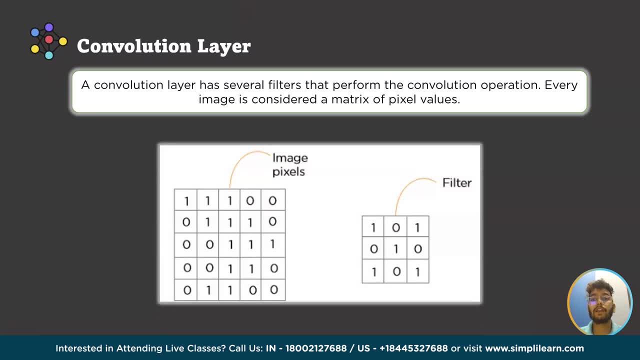 So this is the first step in the process of extracting valuable features from an image. A convolutional layer has several filters that perform the convolutional operations. every image is considered as a matrix of pixel value. So consider this, the following 5x5 image whose pixel values are either 0 or 1.. 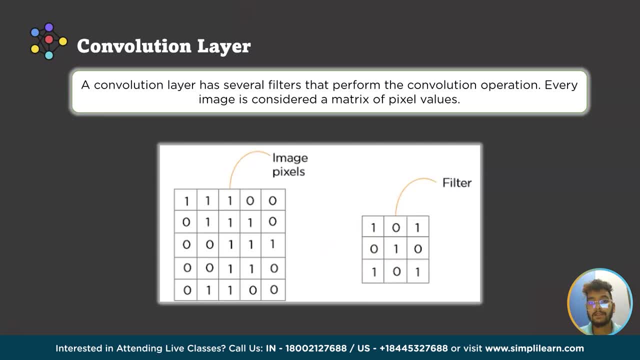 There is also a filter matrix with a dimension of 3x3.. Slide the filter matrix over the image and compute the dot product to get the convolved feature matrix. So this is the first step in the process of extracting valuable features from an image. 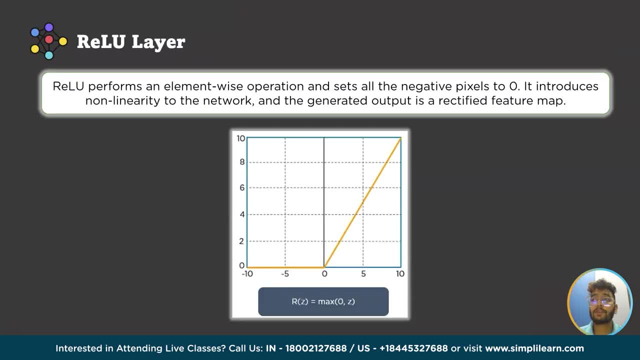 The second is ReLU layer. ReLU performs an element-wise operation and sets all the negative pixels to 0. It introduces non-linearity to the network and the generated output is a rectified feature map. So below is the graph of ReLU function. 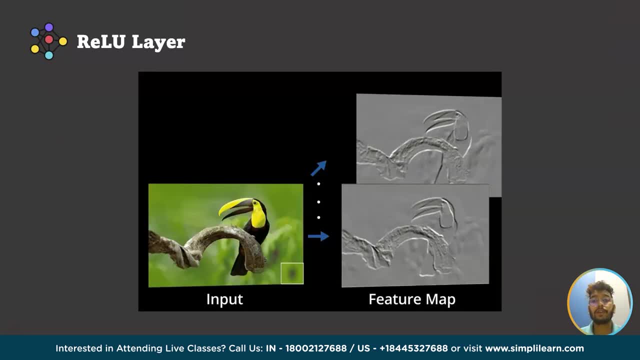 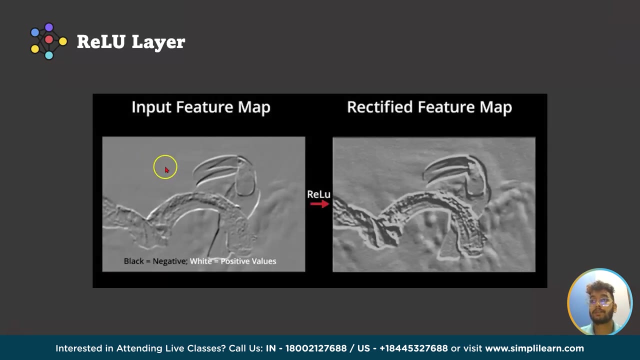 So the original image is scanned with multiple convolution and ReLU layers for locating the features Like this. ReLU layer creates the feature maps like this and after that input feature map creates the rectified feature map. This is how black negative equals white non-negative values or positive values. you can say: 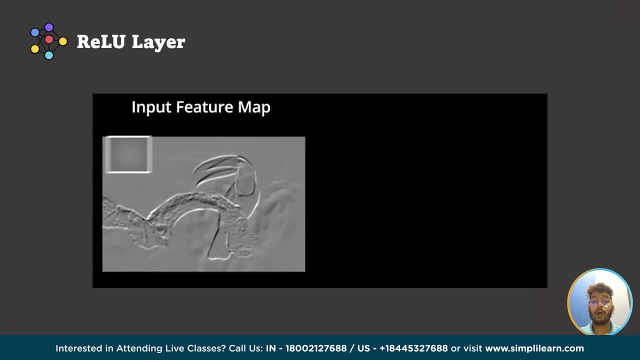 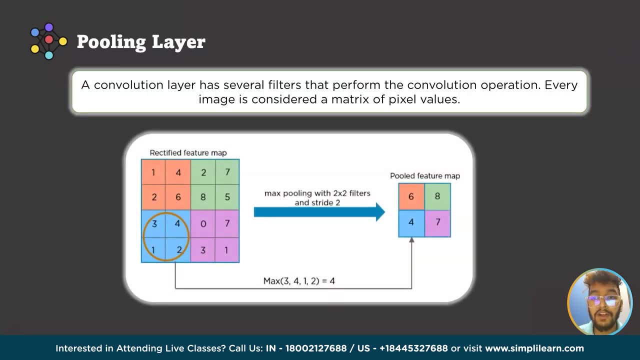 So it will create the rectified feature map, ReLU layers. So now third layer comes into the action: pooling layer. So pooling layer Pooling is a downsampling operation that reduces the dimensionality of the feature map. The rectified feature map now goes through a pooling layer to generate a pooled feature. 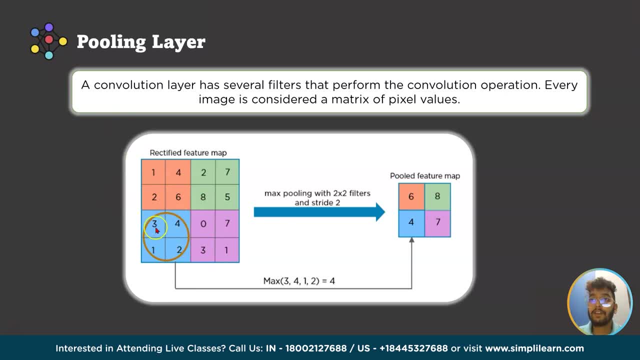 map. So this is a rectified feature map. So here 3,, 4,, 1,, 2.. From this it will take the maximum value. Here is 4, and from this it will take the maximum value 7 and from this it will take the 8 and. 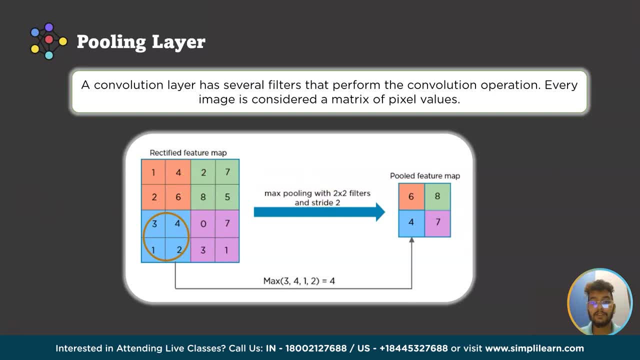 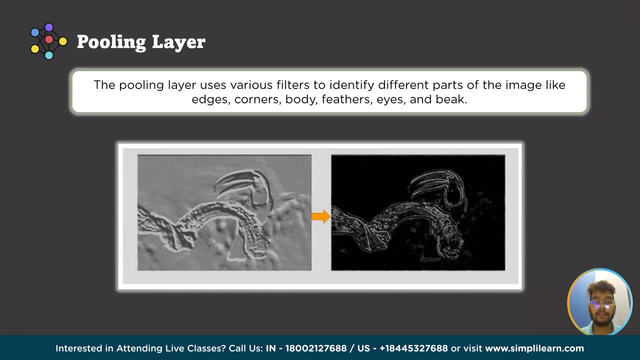 6.. Okay, So max pooling with 2 by 2 filters, and this is the stride 2.. The pooling layer uses various filters to identify different parts of images, like edges, corners, body feathers, eyes and beak, as you can see from the picture. 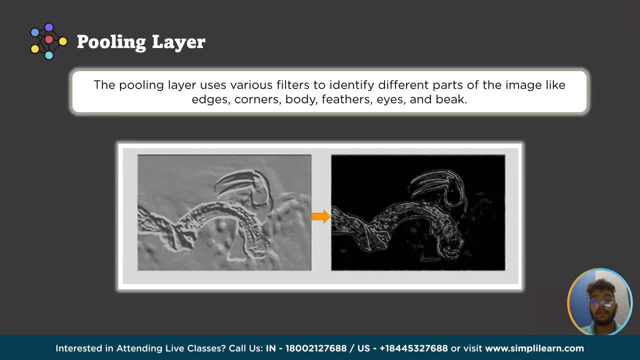 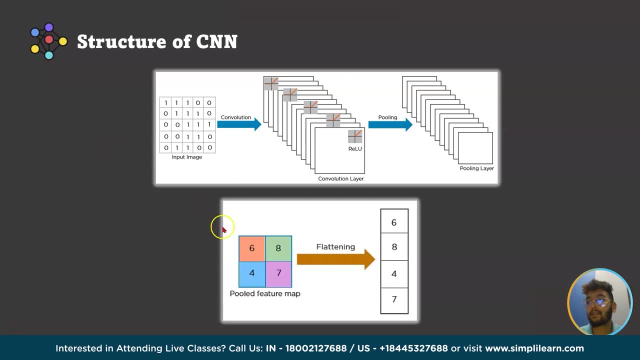 So now let's see how the structure of CNN looks so far. So the diagram represents the structure of CNN so far. So the next step is a process is called flattening. This is called the flattening process, So flattening is used to convert all the resultant two-dimensional array from pooled 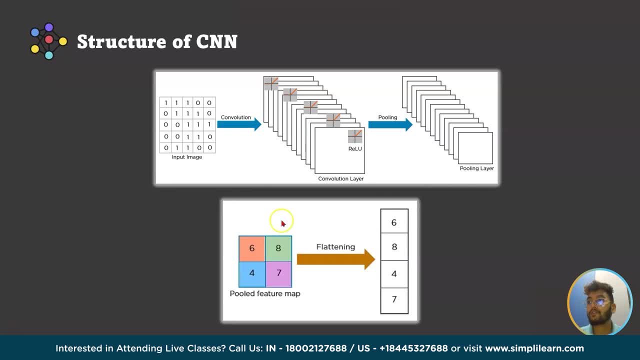 feature maps into a single long, continuous linear vector. So, as you can see, it is a pooled feature map. After flattening it converts into single long, continuous linear vector. The flattened matrix is fed as input to the fully connected layer to classify the images. 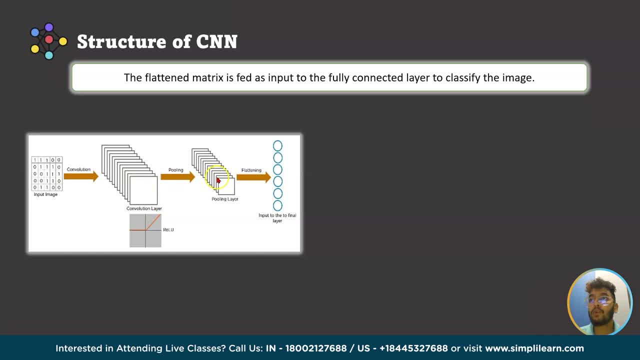 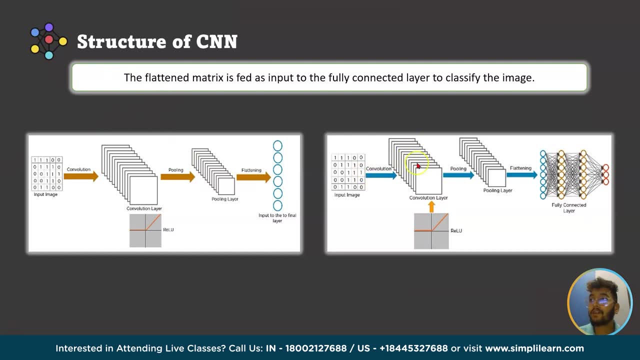 So this is CNN. Here comes the ReLU, Then pooling, Then pooling, Then it is the input to the final layer. After this, So input image, Then convolutional layer, Then ReLU layers comes in. 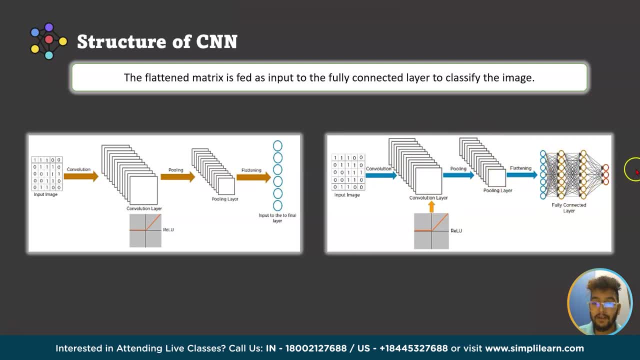 Then pooling layer, Then flattening. Now this is fully connected layer, which is CNN. This is how the CNN grade after connecting the three layers: ReLU, convolutional and pooling layer. So this is how exactly does CNN recognize images? 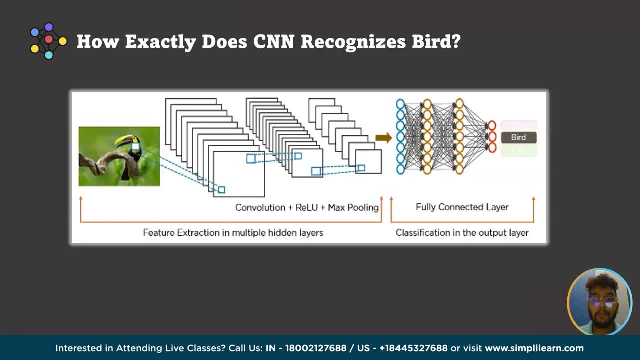 Okay, The pixels from the image are fed to the convolutional layer that perform the convolution operations Here. Then it results in a convolved map. The convolved map is applied to ReLU function Here. the convolved map applied to ReLU function to generate a rectified feature map. 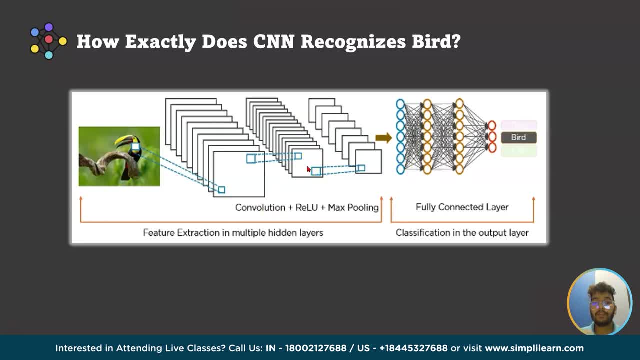 Here it creates the rectified feature map And the image is processed with multiple convolution and ReLU layers for locating the features. Then different pooling layers with various filters are used to identify specific parts of the image. Here the max pooling does. 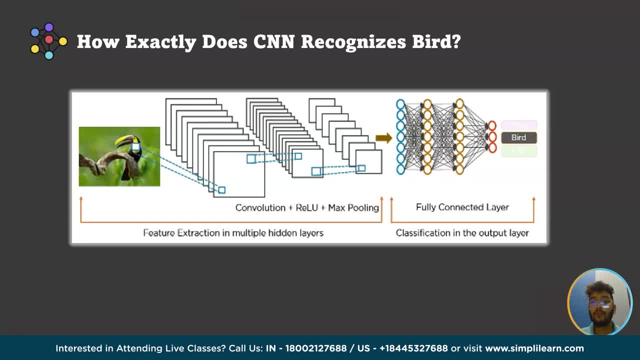 So the pooled features is flattened and fed to fully connected layers. to get This is the pooling Flattened, fed to fully connected layers. This is fully connected layer And that is how it got the final output bar. Okay, This is a feature: extraction in multiple latent layers. classification in the output. 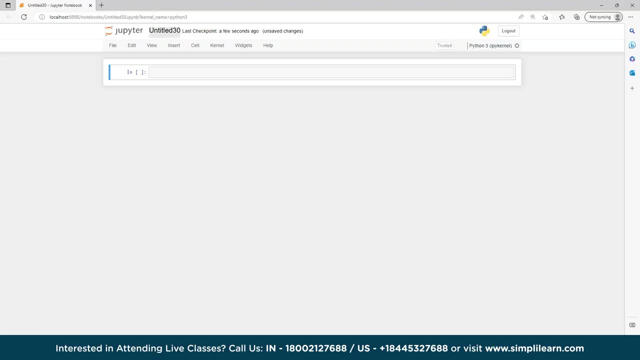 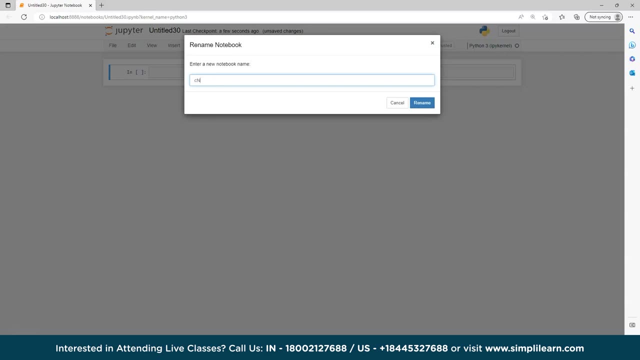 layer. So now, moving forward, let's start the programming part. So here. So this is the Python kernel file. So here, first, we will change the name CNN: CNN For Pignut. 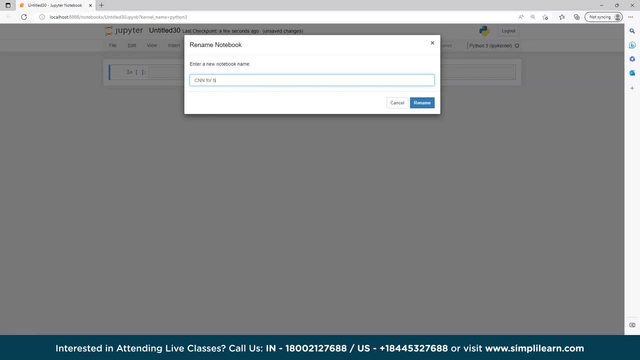 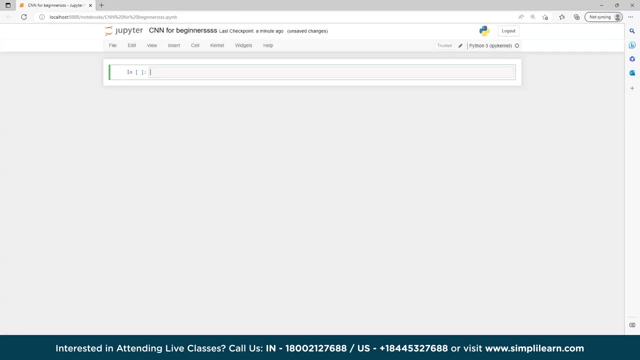 For Pignut, For Pignut Pignus. Okay Then, Okay, Yeah, so first we will import some major libraries of Python, So I will Write import numpy as np. So you will have to get pgnus and gnius in Python work. 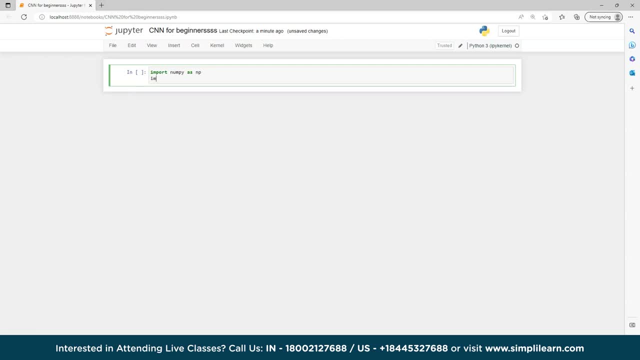 np. then i write: import panda as p and import matplotlib dot pyplot as plt. import cborn as sns, then import keras. after that import tensorflow dot keras. so numpy is a python library used for working with arrays. it also has a function for working in the domain of. 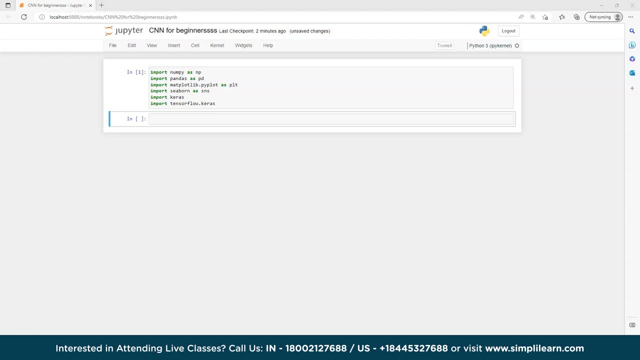 lineal algebra and matrices. it is an open source project and you can use it freely. numpy stands for numerical python and the second one is pandas. pandas is a software library written for Python and Python is a software library written for Python and Python for the Python programming language for data manipulation and analysis. in particular, it 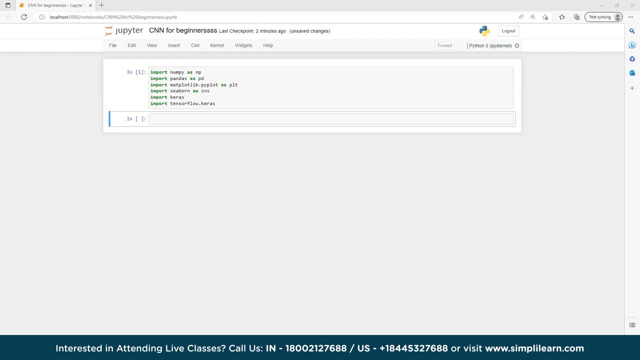 offers data structure and operations for manipulating numerical tables and time series. and the third one is matplotlib. so for python and its numerical extension, numpy, matplotlib is a cross-platform data visualization and graphical charting package. as a result, it represents a strong open source subrata for matlab and the API application programming. 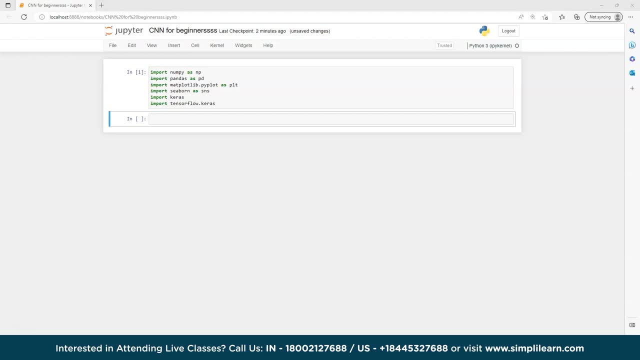 interfaces format: upload: liv allows programmers to incorporate graphs into gi applications. the fourth one is murdered command division, which is a non standard open source activity doc emulatorData plot library which does anegree job in dida implementation and 할 host causation. The fourth one is Seaborn. Seaborn is a Python data visualization library based on Matplotlib. 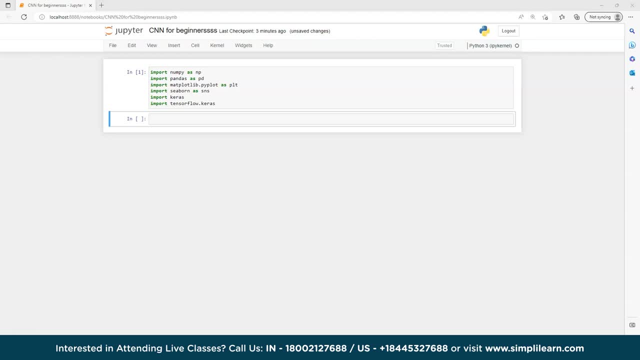 It provides a high-level interface for drawing attractive and informative statistical graphics. For a brief introduction to ideas behind the library, you can read the introductory notes for the paper And the Keras. Keras is an open-source software library that provides a Python interface for 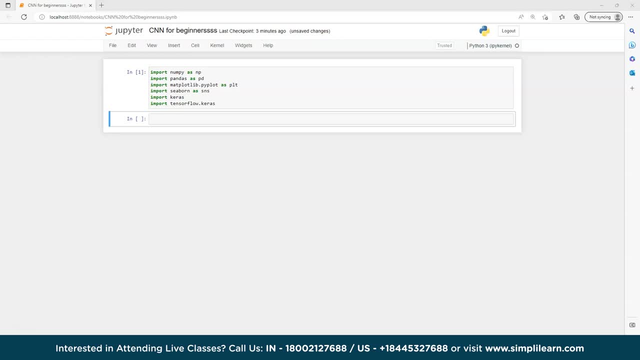 artificial neural networks. Keras acts as an interface for the TensorFlow library. until version 2.3, Keras supported multiple backends, including TensorFlow, Microsoft Cognitive Toolkit, Theano and PlayDML, And the fourth one is TensorFlow. TensorFlow is a free and open-source software library. 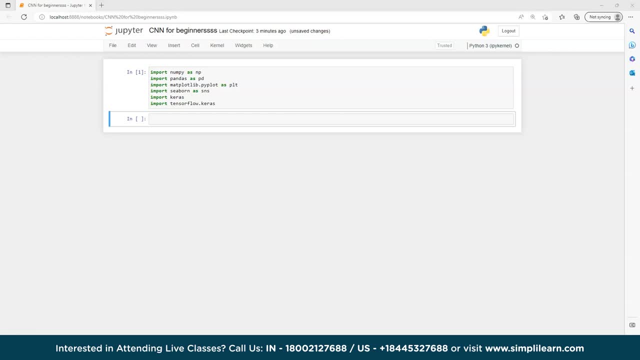 for machine learning and artificial intelligence. It can be used across a range of tasks, but has a particular focus on training and inference of deep neural networks. Okay, So here we are going to load data. First let me write a line: Xtrain, ytrain, xtest, ytest, kerasdatasetsfession- mnist, mnist, mnist, mnist, mnist, mnist. 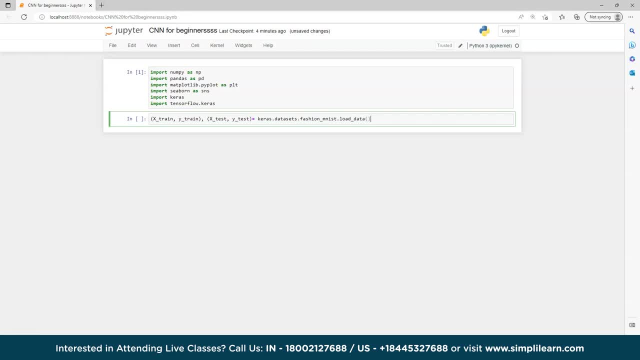 dotloaddata. So there are ten different classes of images for a library, Like t-shirt, top, trouser, pullover, dress, coat, sandal shirt, sneaker, back ankle boot, etc. And the images that I mentioned are 28 by 28.. So in this we are splitting the data into 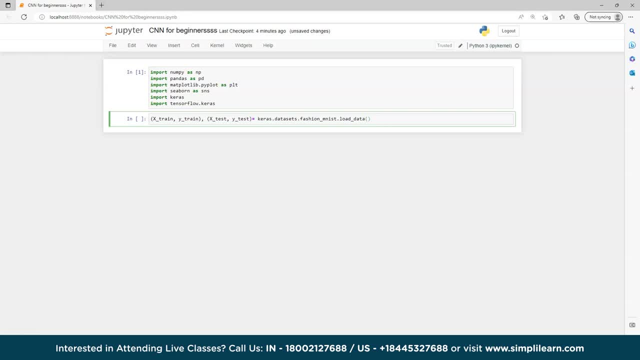 training and testing sites. So what is mnist? So fashion mnst consists of 60,000 training images and 10,000 testing images. So fashion mnist consists of 60,000 training images and 10,000 testing images. It is the. 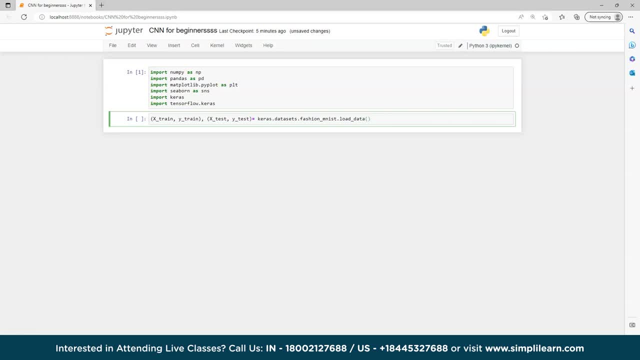 mnist like fashion product data. The developers believe MNST has been overused, so they created this as a direct replacement for the dataset. Each image is in grayscale and associated with a label from 10 classes. Each image is 28 pixels in height and 28 pixels in width, for a total of 784 pixels in total. 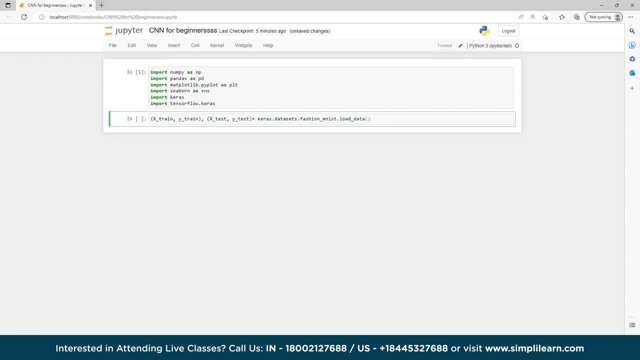 So each pixel has a single pixel value associated with it indicating the lightening or darkness of that pixel, With higher number meaning darker. the pixel value is an integer between 0 and 255.. So, moving forward, we will see that how much data we have in training and the rest. 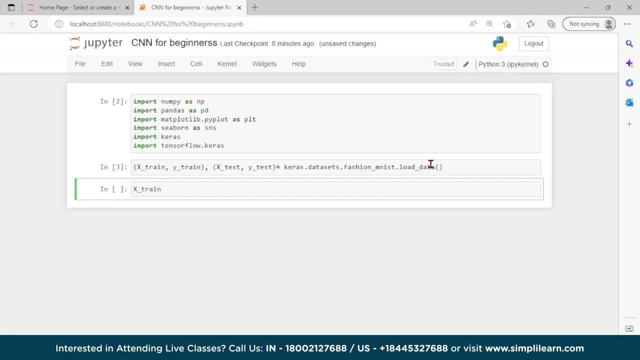 So here I will write Xtrainshape. there is no need, I guess, for this Xtrainshape, Ytrainshape. see, we have 60,000 rows and 28 columns for a particular dataset. Now, Xtestshape, Ytestshape. 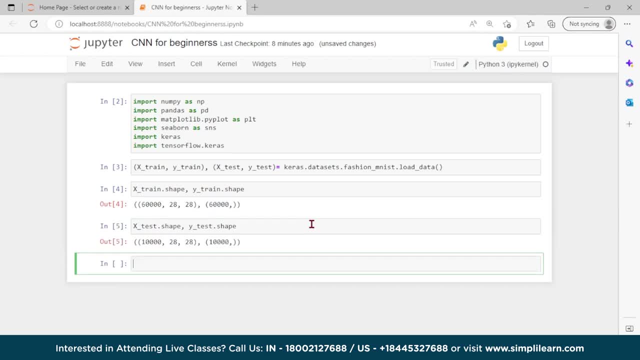 Okay, Okay, There are in the testing. we have 10,000 rows and 28 columns. I already told you before when I talked about the dataset. we have 60,000 training images and 10,000 testing images. 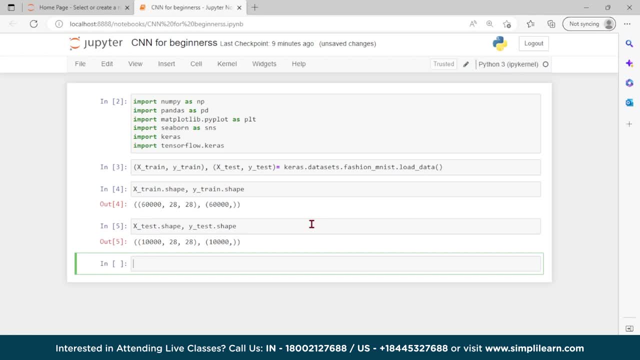 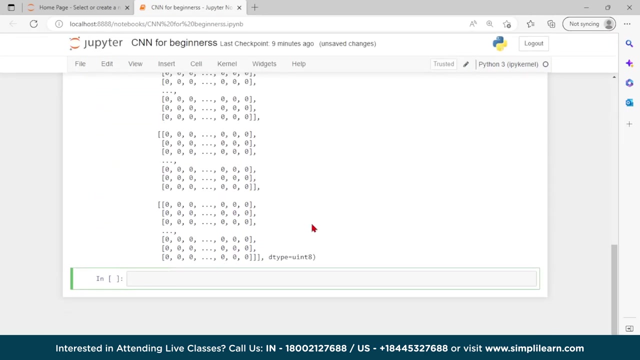 Okay So, and if you want this full code, I will provide you in the description box below. Just comment, for the same, that you want the full code. Okay So, now let's train the data. Okay, Then. Xtrainshape, Xtrainshape, Xtrainshape, Xtrainshape, Xtrainshape, Xtrainshape, Xtrainshape. 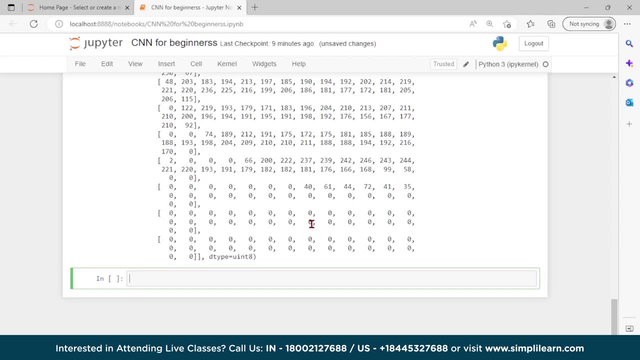 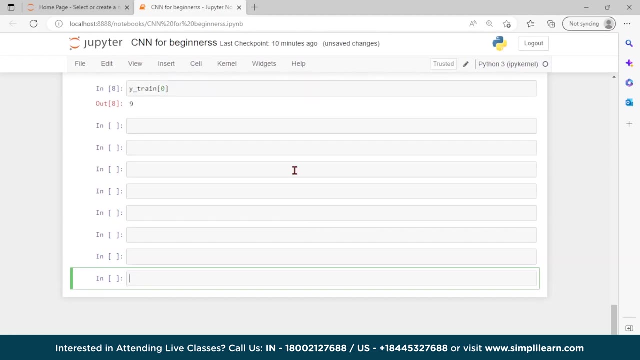 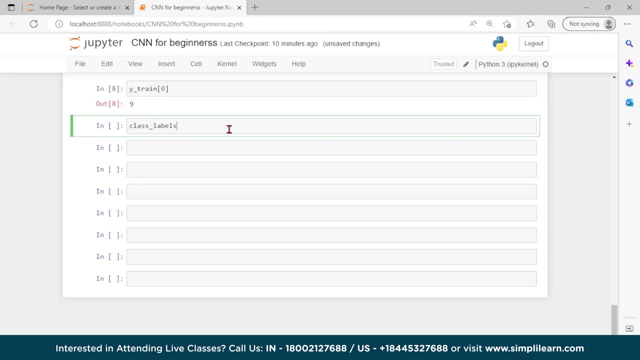 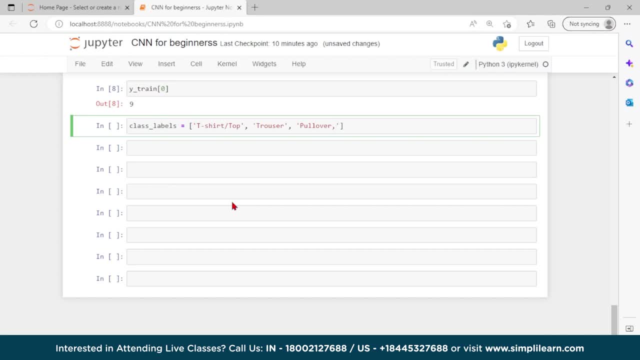 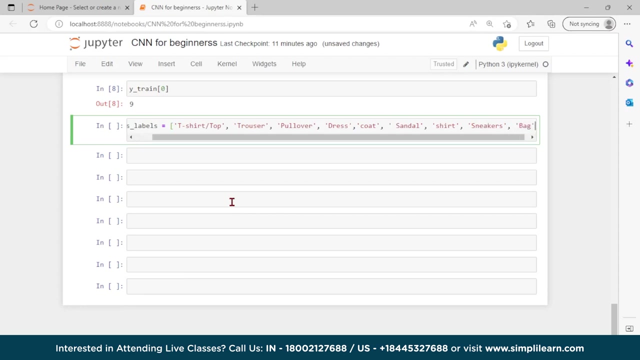 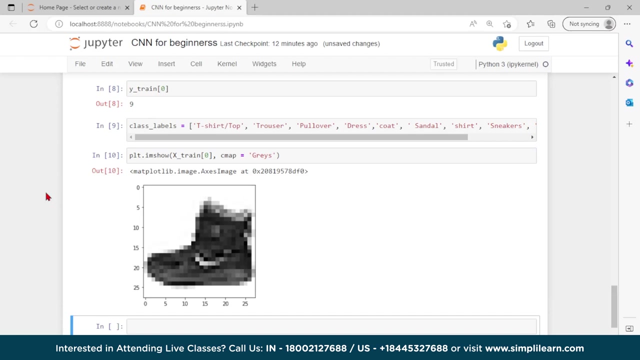 dress, then coat, then sandal coat, sneakers, then bag, ankle boot. let's see some images. so what here? here I will write class, no, no, no, I will write. pltshow show, next train comma: cmap show: great, so see, it is a ankle boot, it looks like an ankle boot. 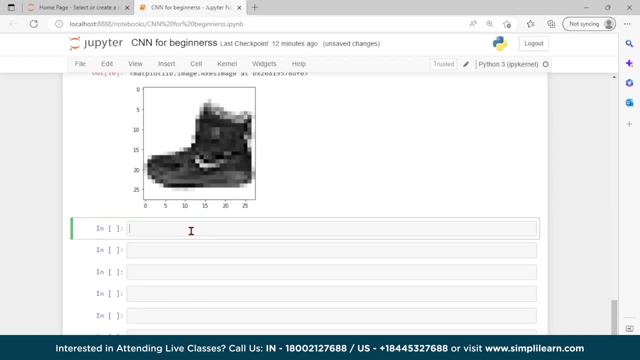 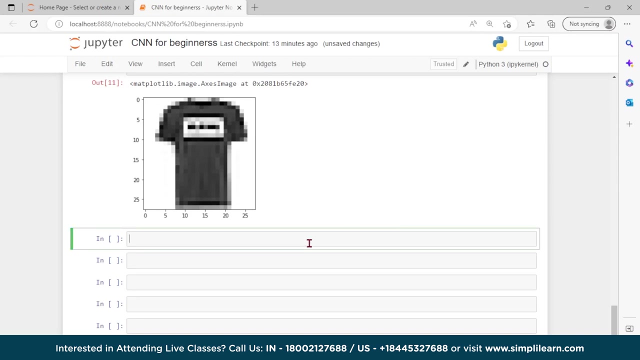 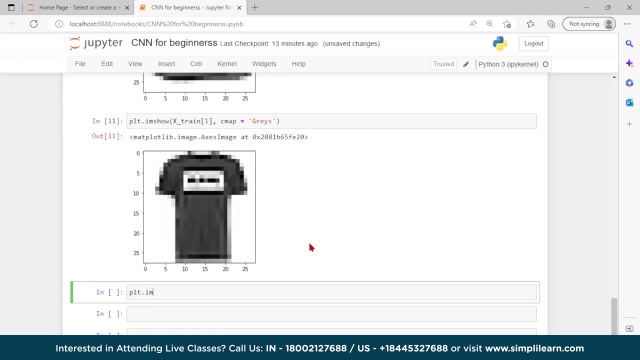 let's see one more plt dot. I am show strain e-map. it is a t-shirt. we have sixty thousand images in the training set so we can check the any. let's see one more PLT dot. I am show strain 15. let's do grace. 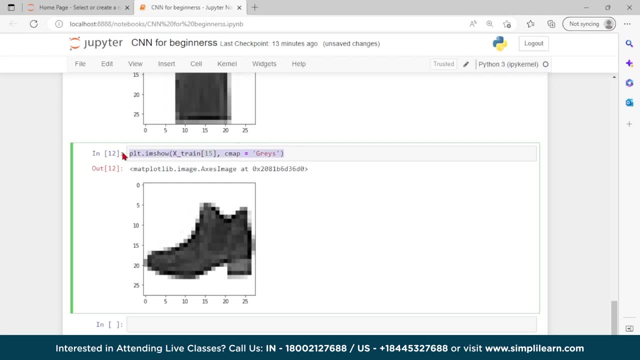 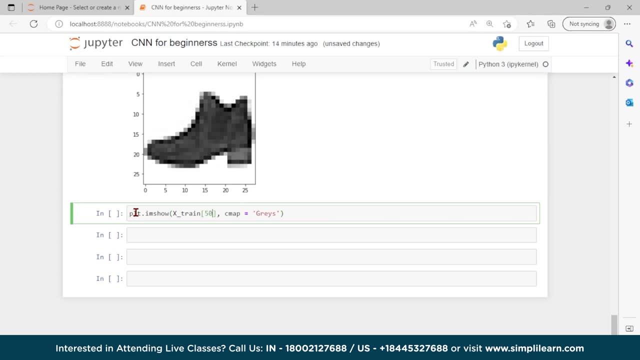 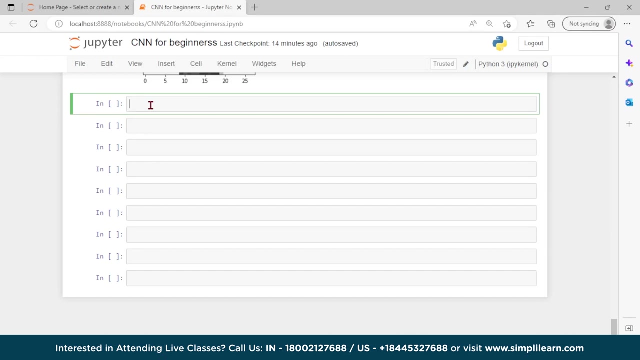 there's a shoe, okay, let's copy it. the last we are checking for the 50 something dress. okay. so this is a for the training. that is why we are writing here x-train, right. so now let's see the all the categories. okay, like sneaker, ankle boot, coat and t-shirt. 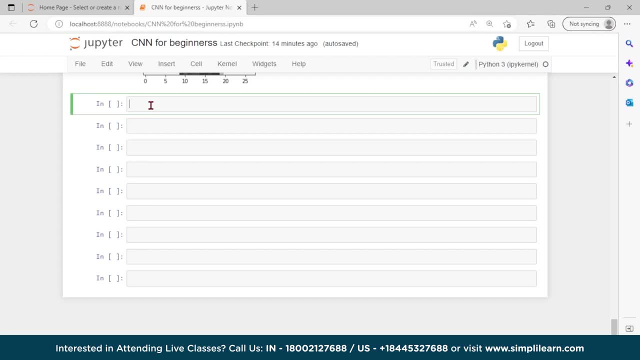 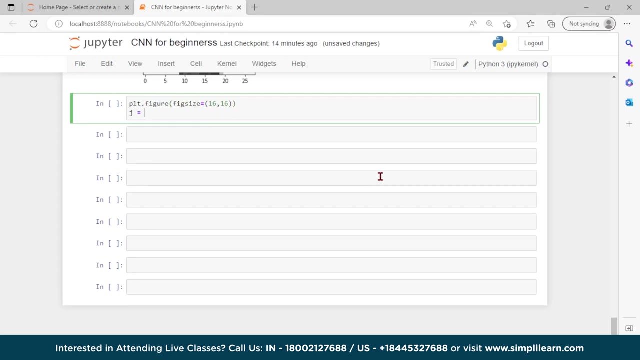 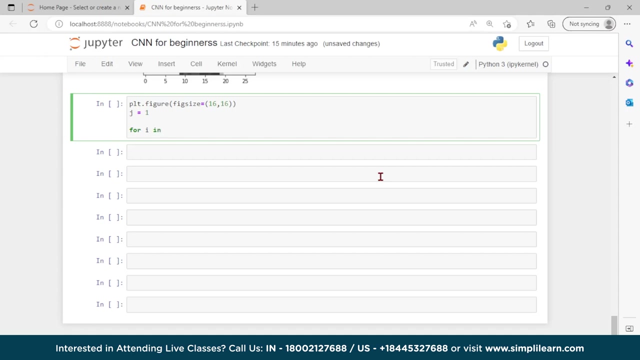 okay, sandal and all. so for the training we are writing here x-train, for that I will write here VLT dot bigger the size, I will give 16 by 16 a, it was 21 for I in and P dot random but rent in. 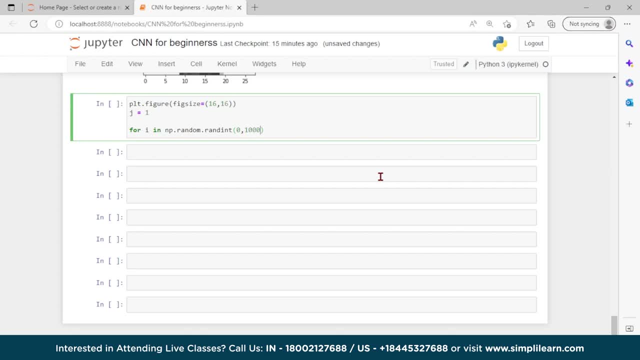 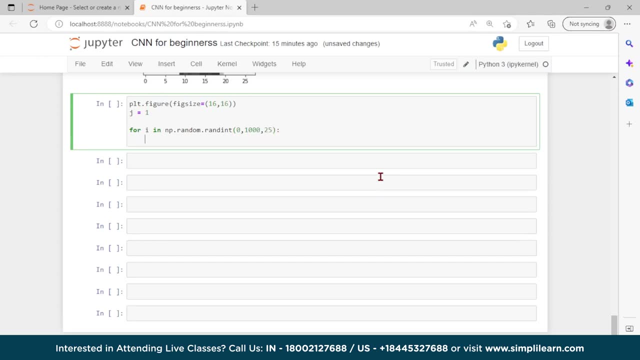 you know, come on 10,000, 30,000, only 25 LD dot subplot. you know, come on 10,000, 30,000, only 25 VLT dot subplot. you know, come on 10,000, 30,000, only 25 VLT dot subplot. 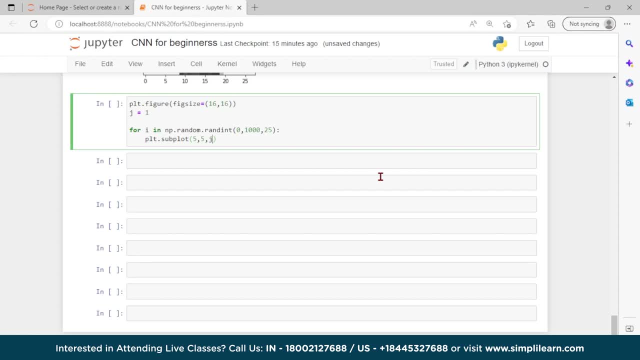 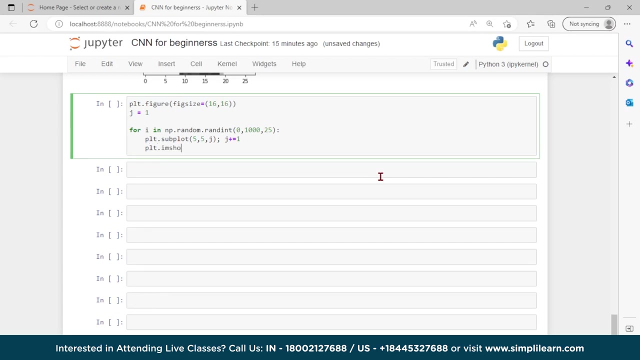 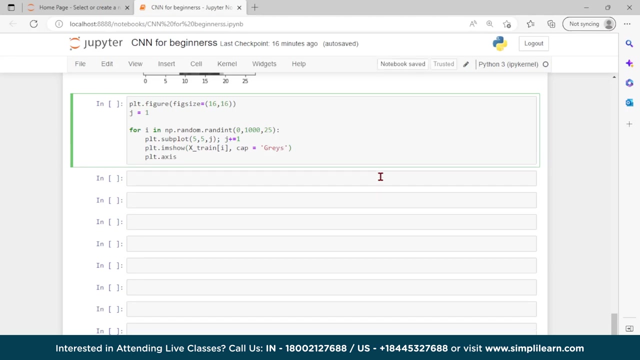 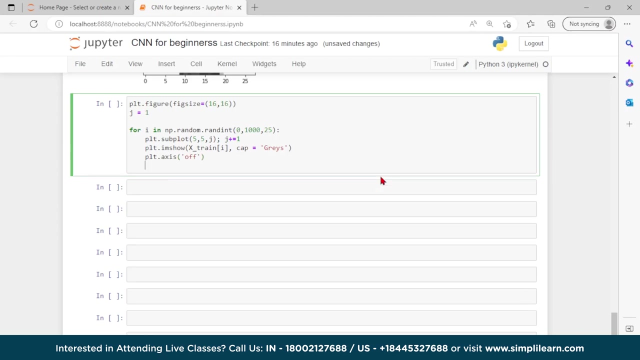 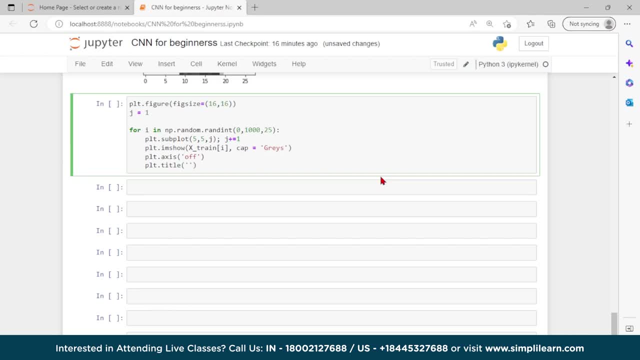 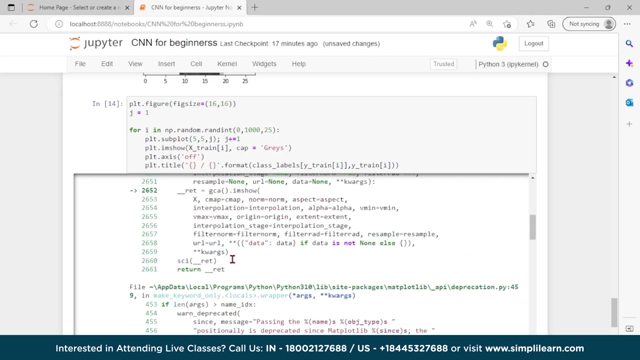 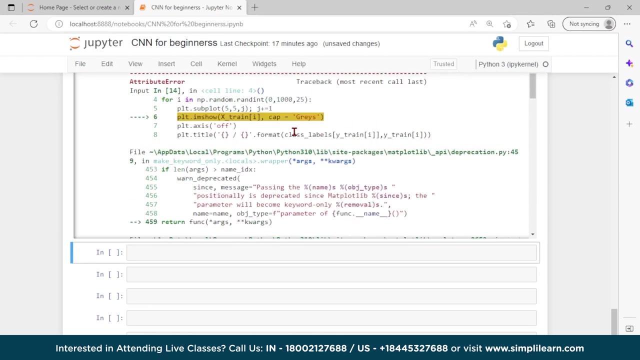 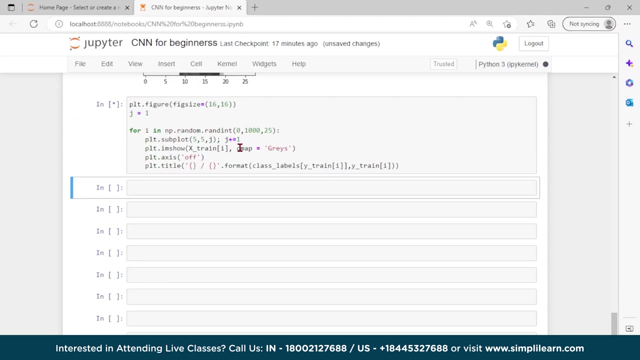 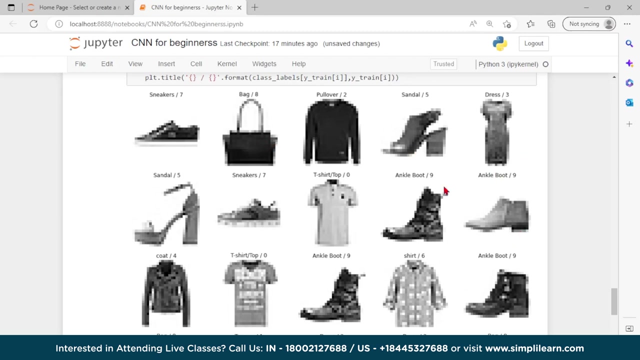 again calibrations what i will write here: dot format as pulse: y train: one white train: okay. so now let's see run it. okay, so there is an error. object has no property cap: okay. okay, it is c map. okay, now you can see the sneaker bag, pullover, sandal, dress. so all the categories okay. shirt. 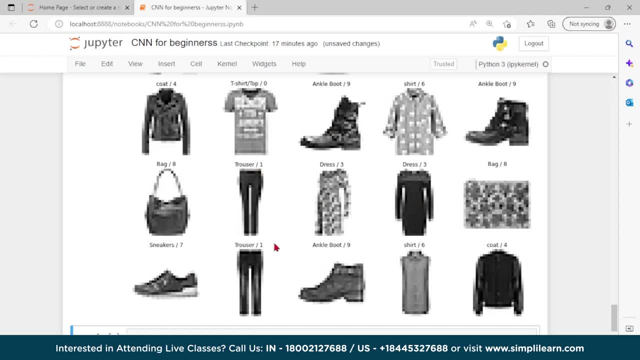 coat, bag, sneaker- this is for the training- the trousers. we are training all the images- okay, for the model. so now, what do you need to do? okay, so now what we will do. we will reshape some training data- okay, the length and the testing data length. so, moving forward, we will do that. let's. 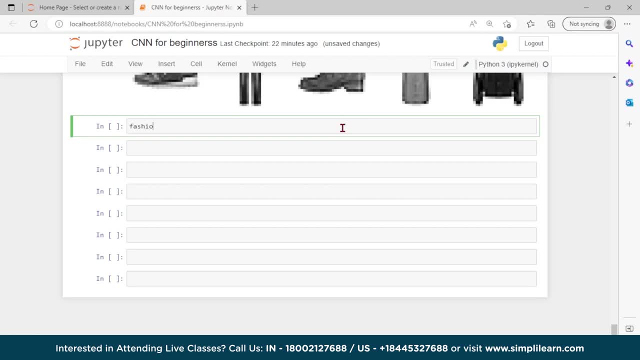 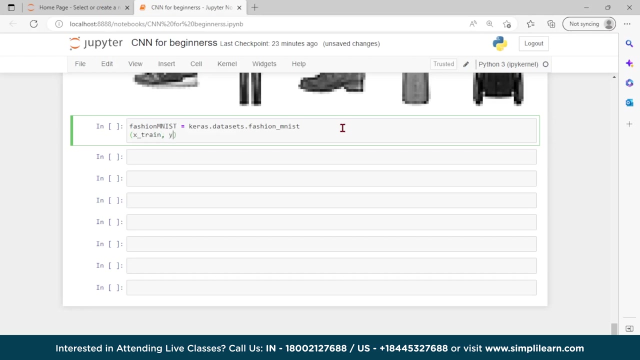 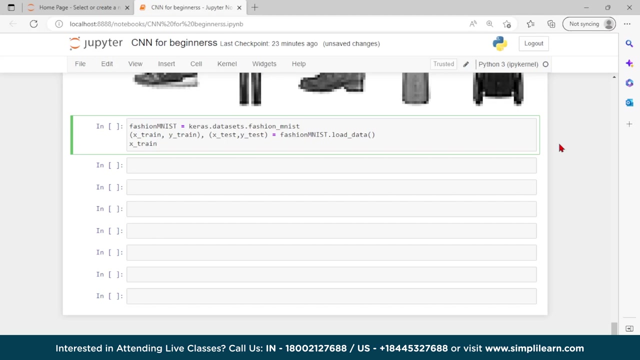 do reshaping and on. So fashion m is to kresdatasetspassion, xtrain, ytrain, xtest, fashion yta, veda, extr m yelled beast, hitata h, these dimensions. so here i will write x train minus one, okay. or we can write x train equals to extend or reshape length extreme, okay. 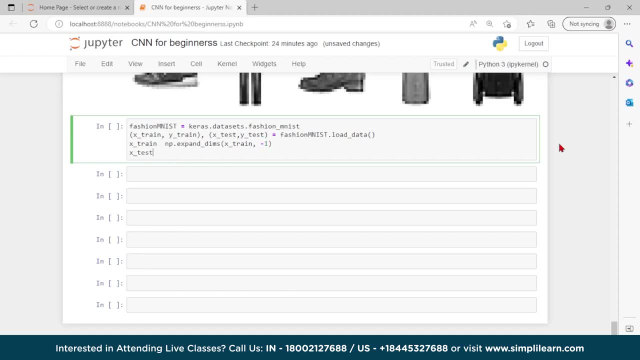 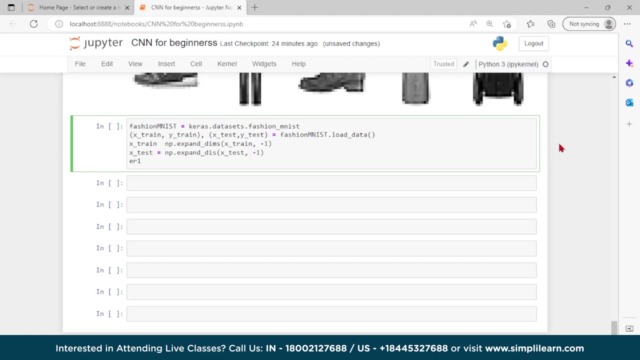 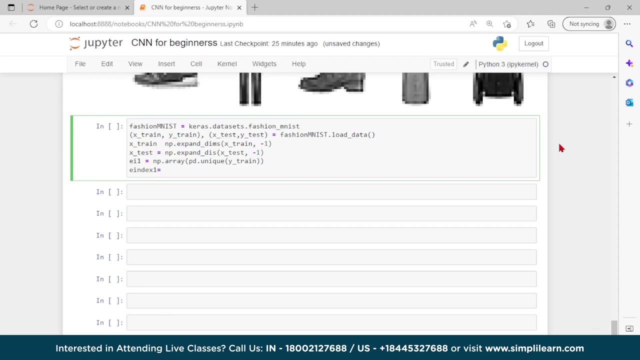 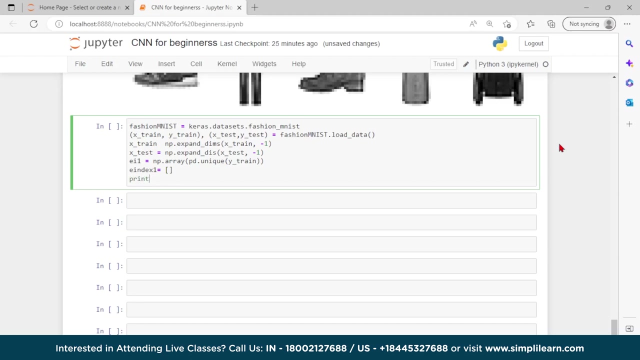 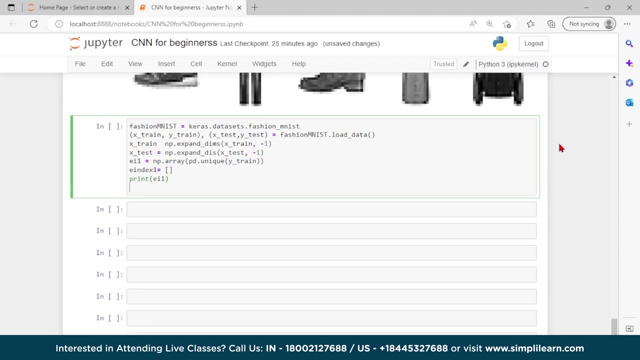 here i will write x, test plus two, and p dot expand dimensions. x test comma minus one. okay, here i will let say one plus two. np dot, add a, d dot unique. and here i will write x, train, x 1 equals to train, train, train, train, train. 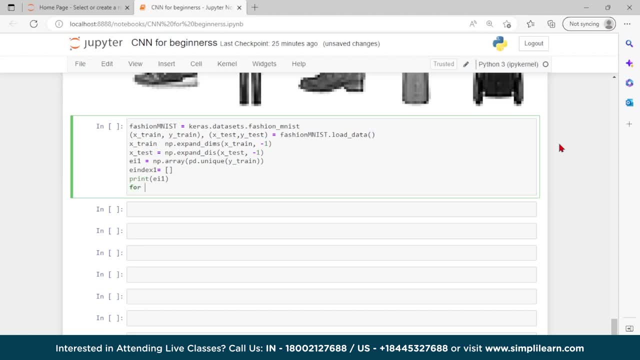 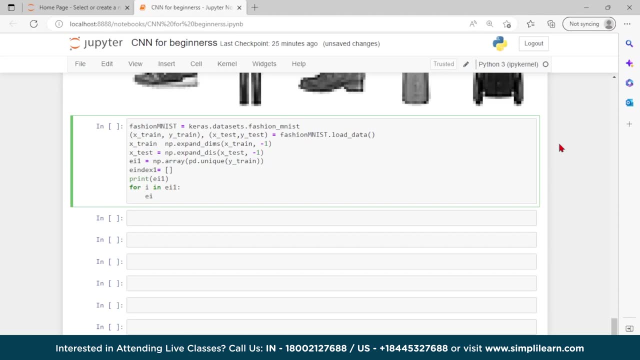 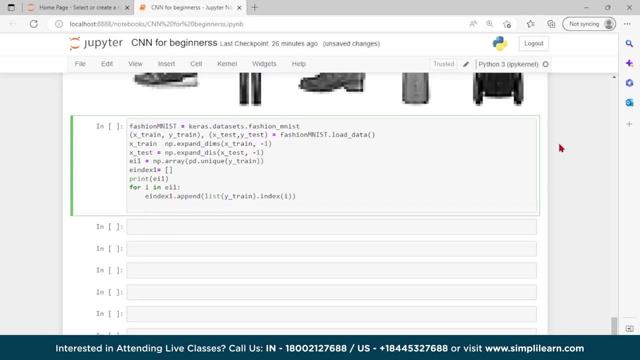 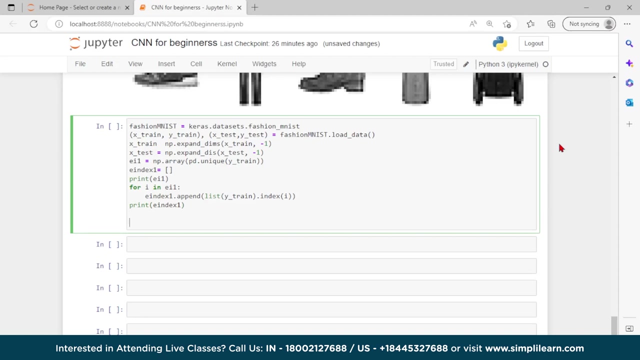 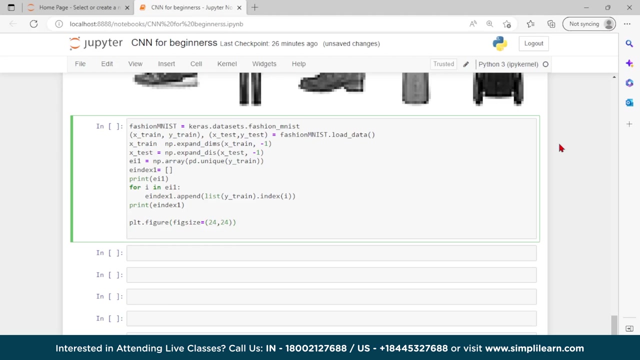 train for a one, then a index one. what append? append to list white rain out and x. okay, then print X one, yeah. so cross-check for I in index, print y train: I ok. cross-check for I, in index, print y train: I ok. so here I will write PLT dot figure because size was to 24: 24. okay for X. 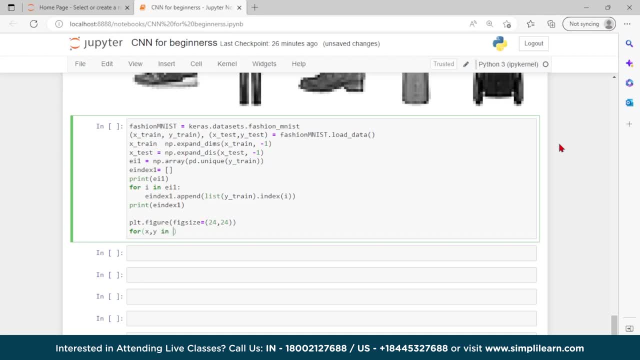 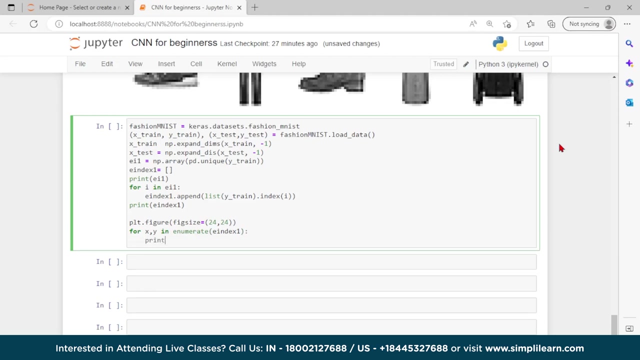 comma Y and enumerate index one. this and I will add print: explain you or ship and PLT dot subplot: who comma five? comma X plus one ELT dot. I am sure answer flow please. and X train. why was to grace plg dot title format a one. 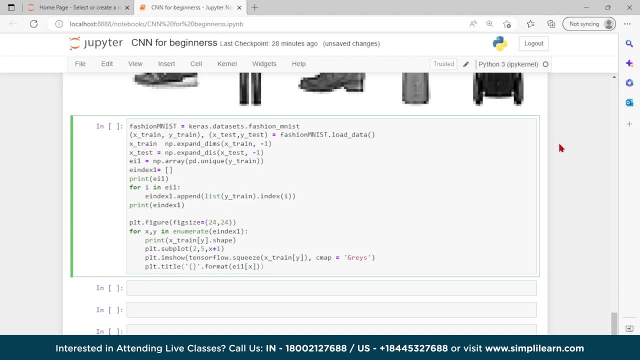 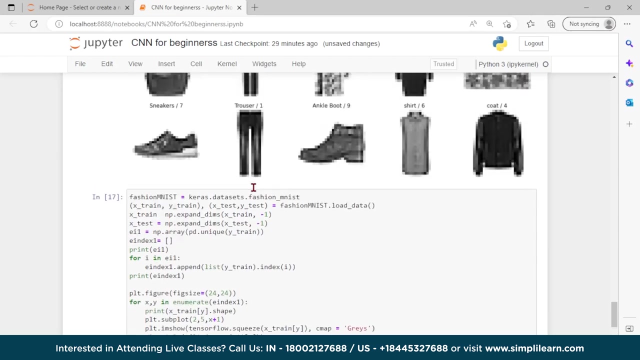 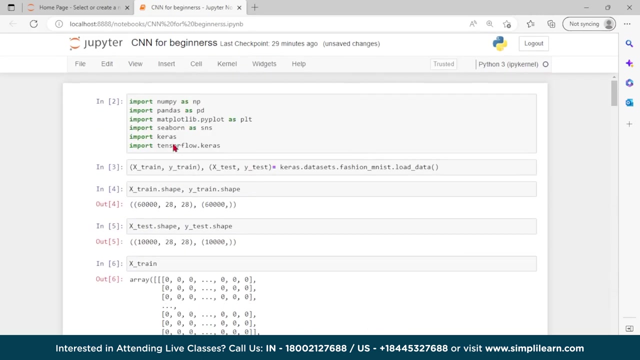 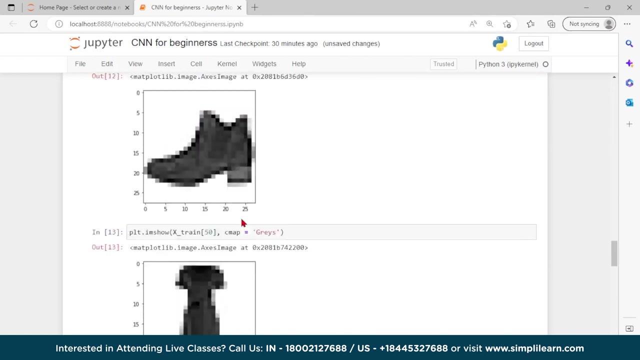 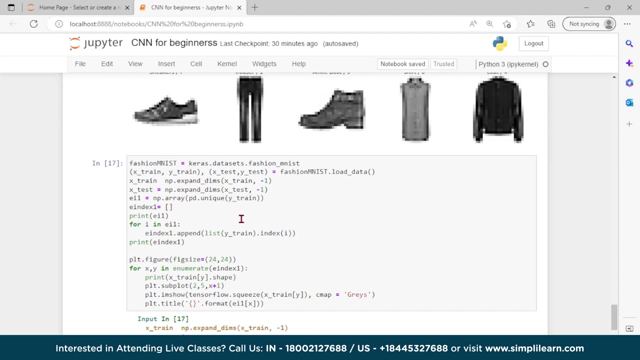 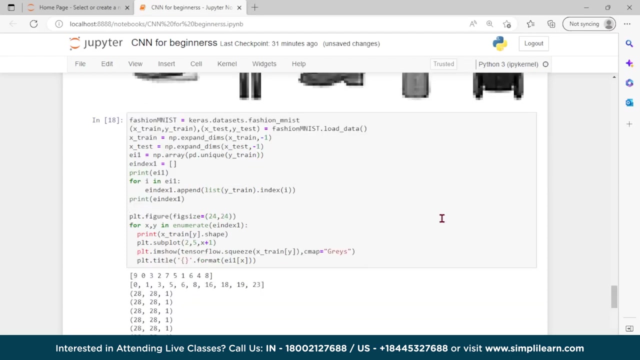 X- okay, x-train and p-dot index. so they expand x-train minus 1: okay, x-train- okay, valid index what I wrote here. let me check import numpy as np. the errors: okay, let me check the others working. these are the 10 category. 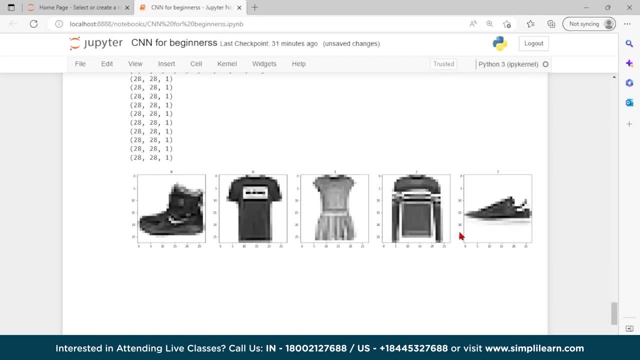 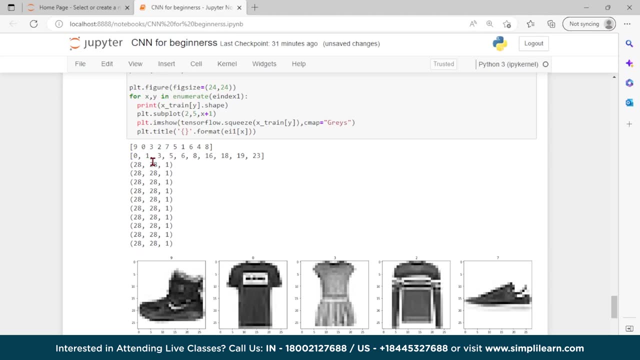 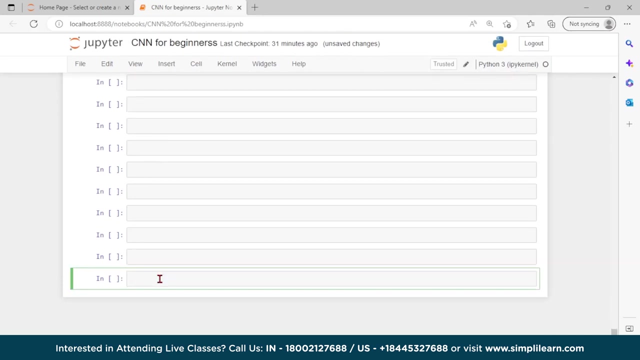 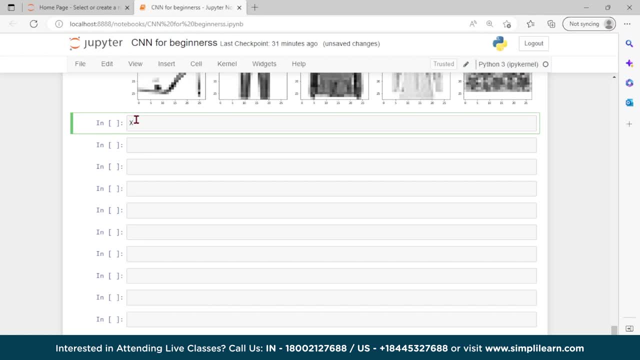 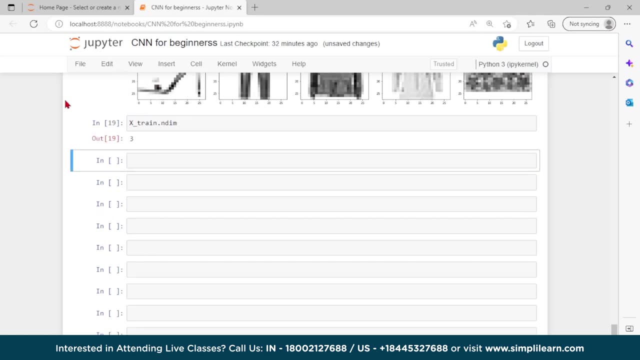 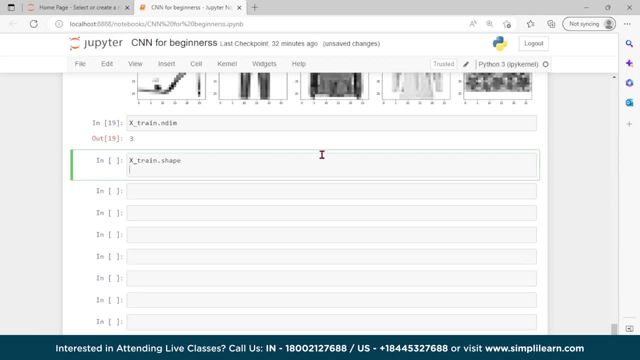 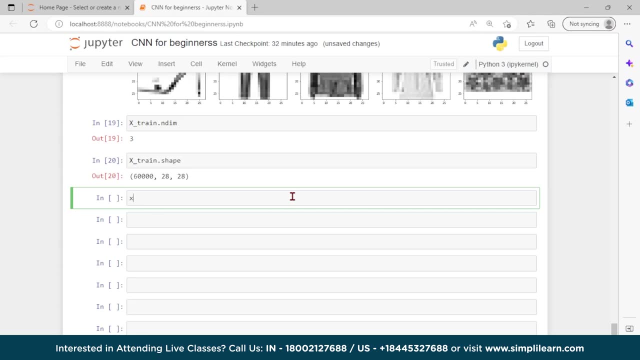 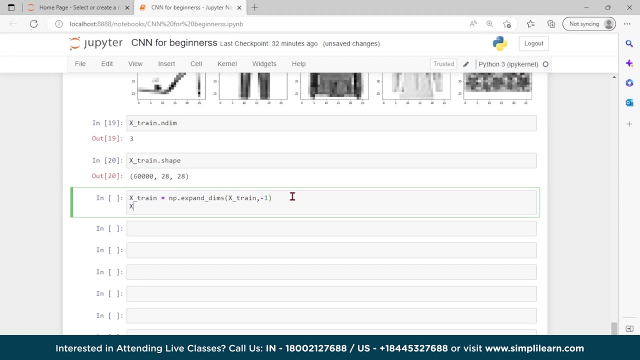 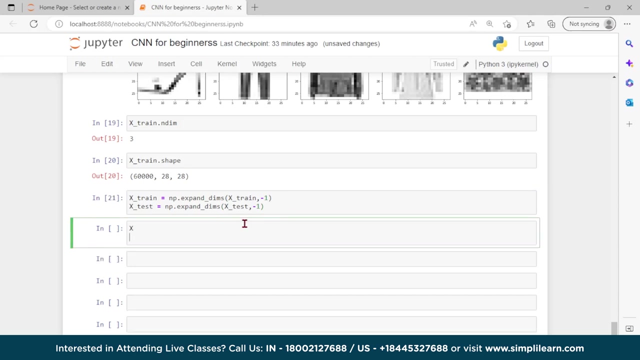 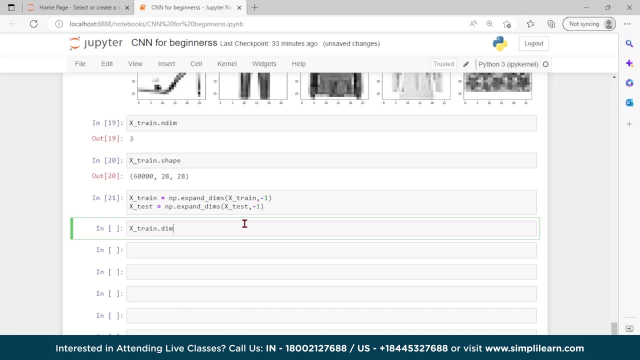 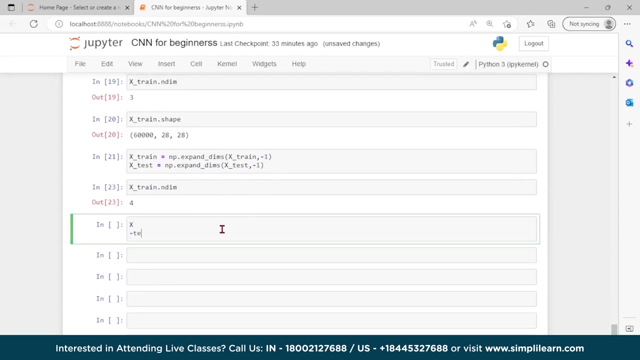 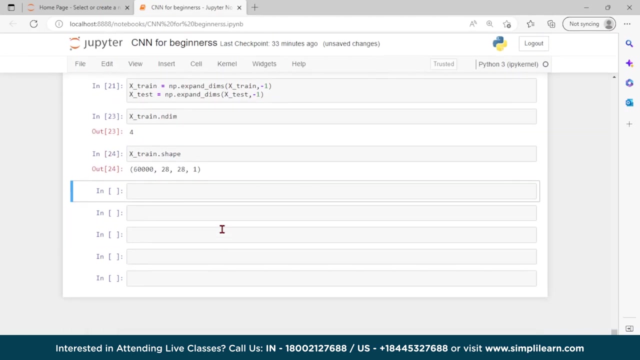 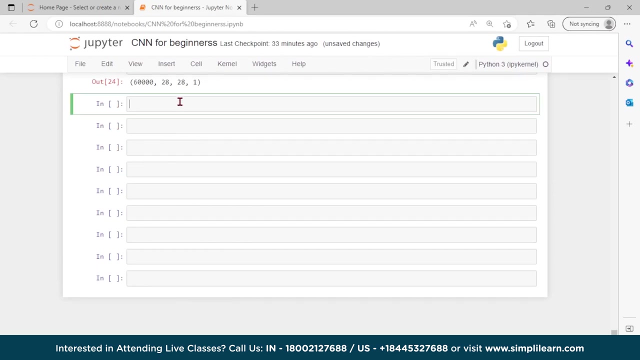 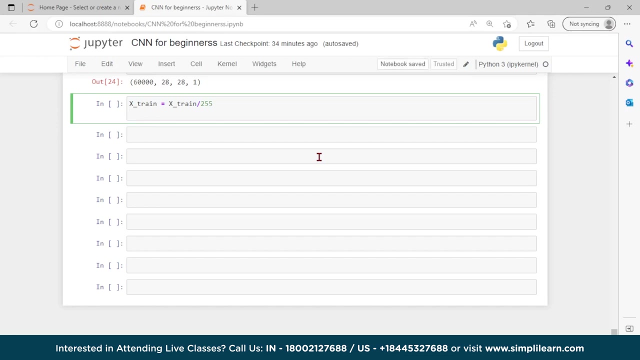 strain and in this is a four-dimensional image. okay, the next strain or shape: okay, fine. so now what we will do, we will do the feature scaling. so for the feature scaling, I will write here: X strain equals to X strain by 255. okay, so here I will write: X test equals to X test by. 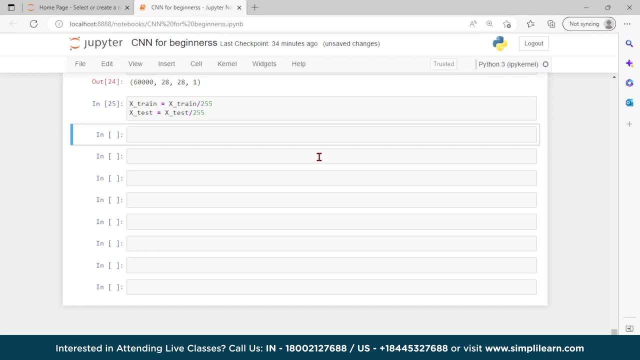 255. so what is feature scaling? feature scaling is a method used to normalize the range of independent variables or features of the data. so in data processing it is also known as the data normalization and is generally performed during the data pre-processing steps. okay, so let's see. the data is in zero to one for that right here, small, small code X. 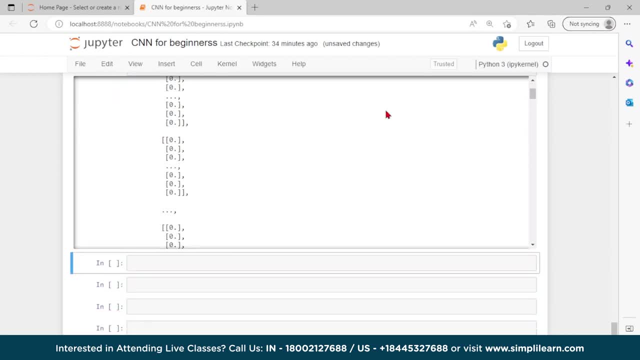 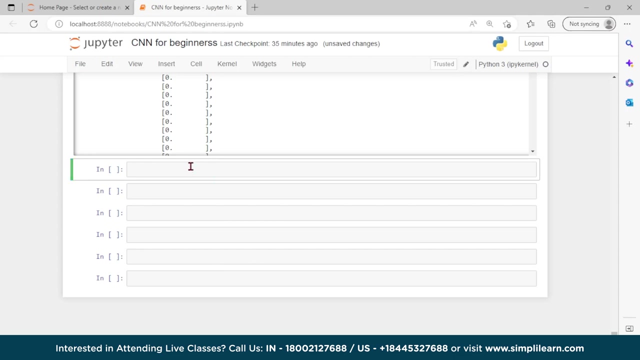 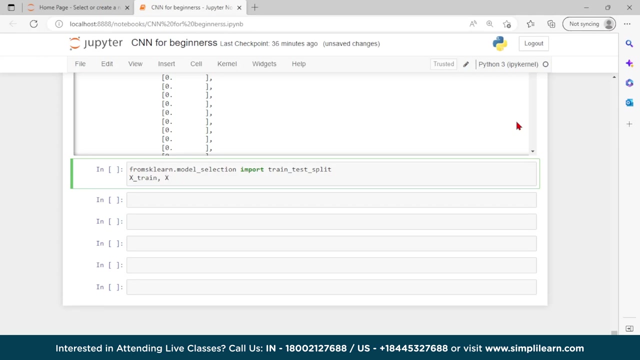 strain and zero. So now what we will do. we will just click the data set for the validation set. okay for that. we will write here from sklearn model you Model Selection: Import Strain Trust, Strain X, Value Y, Train. 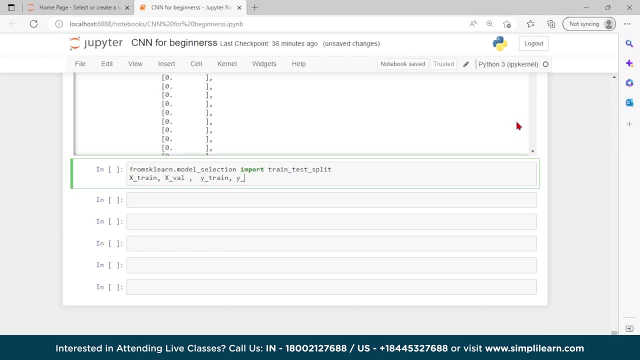 Test Split and here I will write: to enter split. then okay, split. then I will write here: Okay, X Train Y Train Test over here now. I will write: X Train Y Train Test over here now. 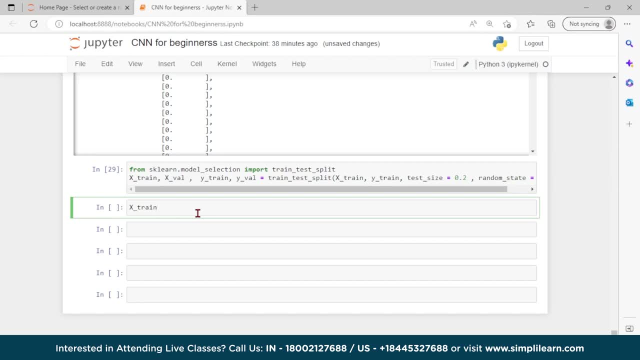 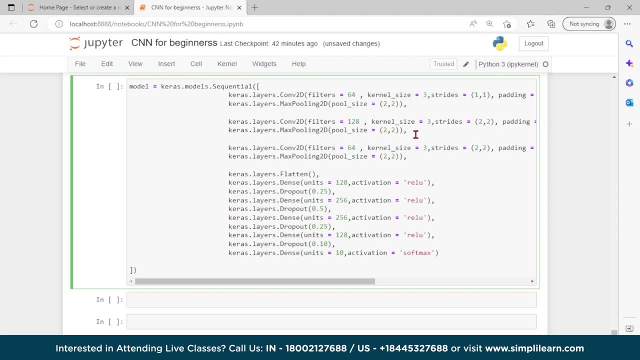 I will write X Train, Y Train Test over here. now. I will write X, Train, Y Train Test over: okay, and there is dense, dense again the layer. so max pooling- here is a term, max pooling 2d, so it is a pooling or max pooling operation which. 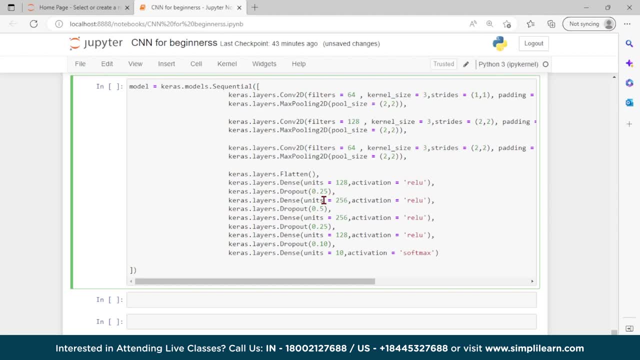 calculate the largest or the maximum value in every pageant and in the every features. okay, so it is used in the pooling operation that calculates the maximum value for the patches and to create the pool feature map. got it, and here is a dense. so dense is like in any neural network. a dense layer is a layer that is deeply connected with. 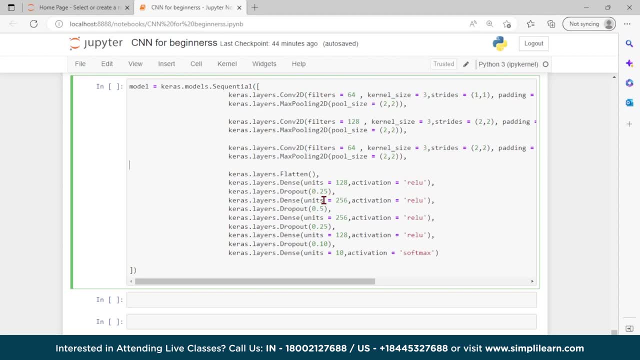 the precision preceding layer, so which means the neurons of the layer are connected to every neuron of its preceding layer. the layer is mostly commonly used in artificial neural network. okay, and there is dropouts, like how much it will be dropout for every you know layers from every layers. 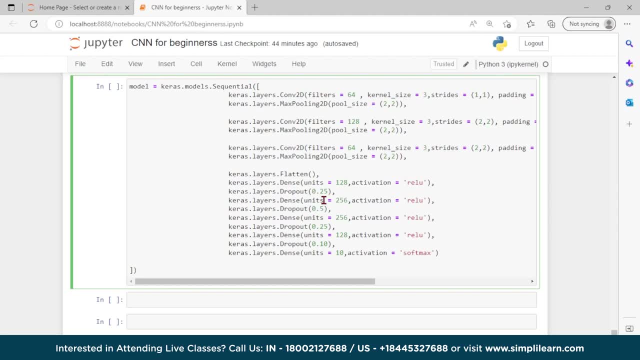 there is one more word: flatten. so flattening is used to convert all the resultant two-dimensional array from paragon to superposition. so what is the flattening that is used to lay out the layers System. and you can see in this example the array is not fully flattened and that is the reason why I am stating it is not fully flattened. 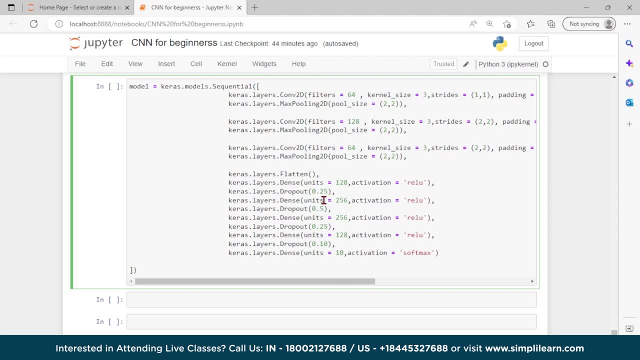 array from pool feature map into a single long, continuous linear vector. the flight and matrix is fed as input to the fully connected layer to the classify image. this, softmax, is a like equation or a function you used to activation function in the output layer of the neural network and that predict a multi 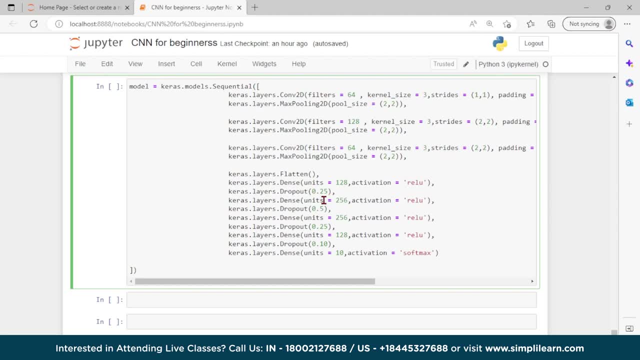 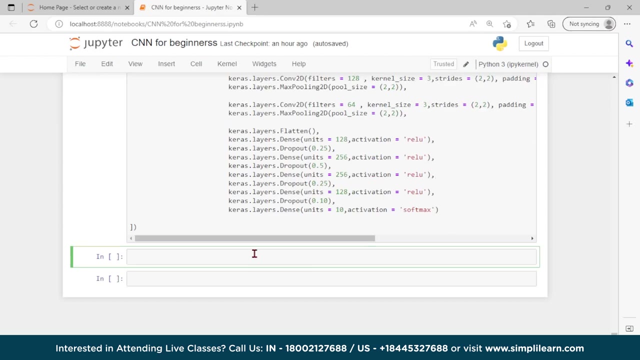 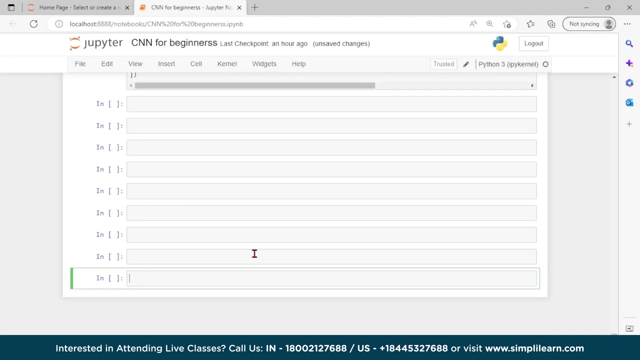 normality, probability distribution, that is, softmax is used as the activation function. okay, and ReLU is again, you know a particular layer, forward the visuals. oh, now what we will do. we will plot the neural network for the workflow. okay, Keras dot, else not modern. well, you file person. 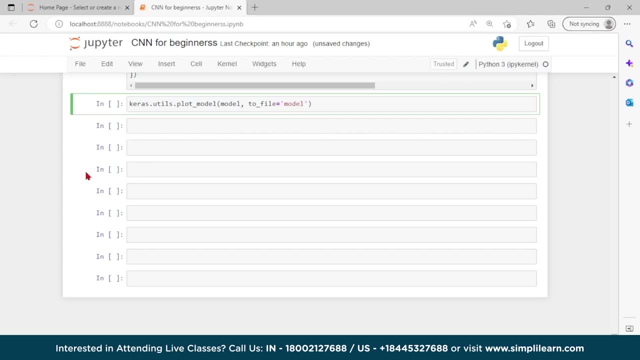 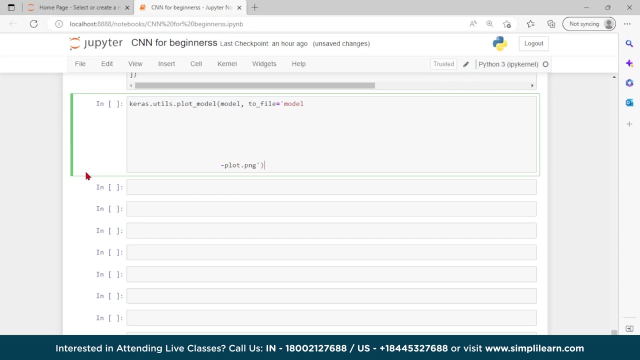 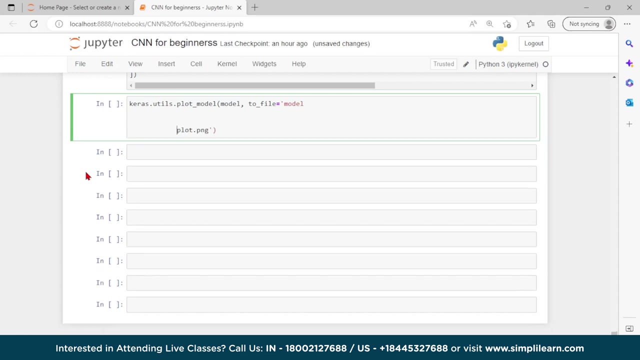 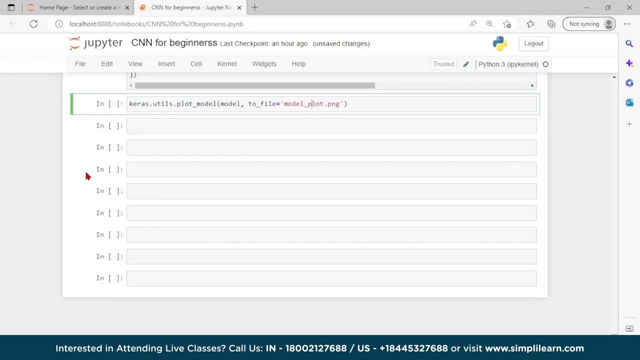 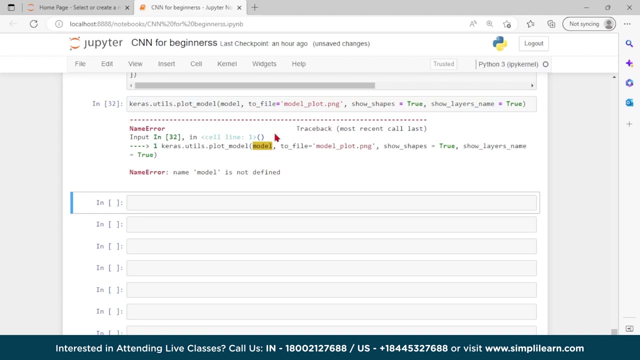 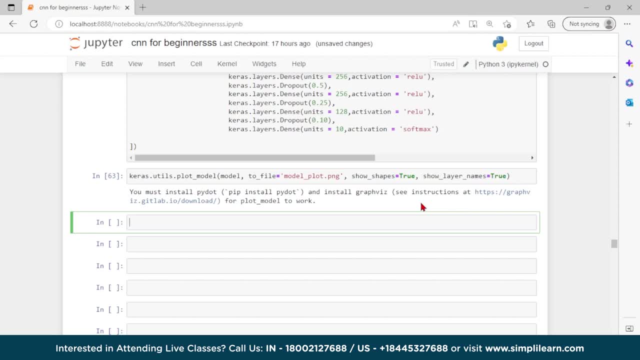 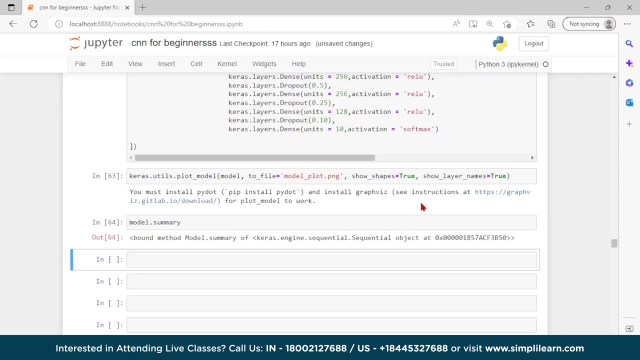 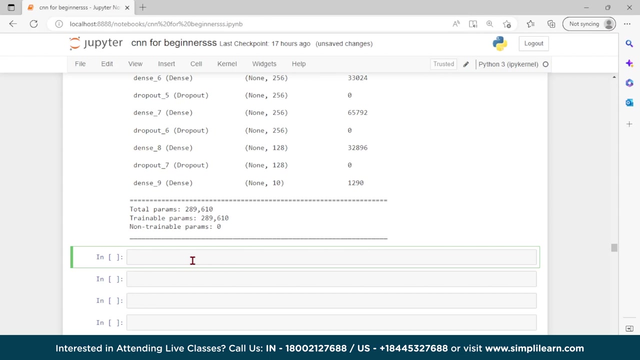 will come back to you. so here what i will try. it will see the model dot summary. this is the model summary. okay, and now what we will do. we will compile and model fitting, do the model fitting. so here i will do the model dot compile optimizer. first two adam. 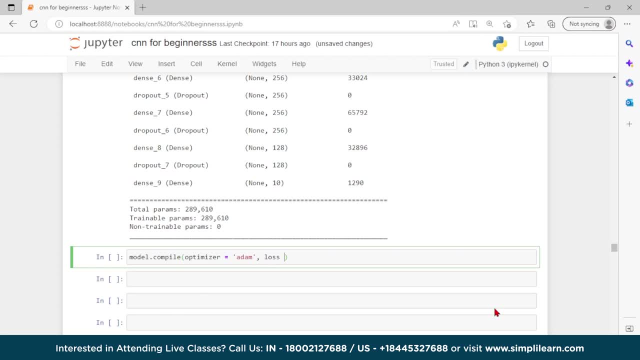 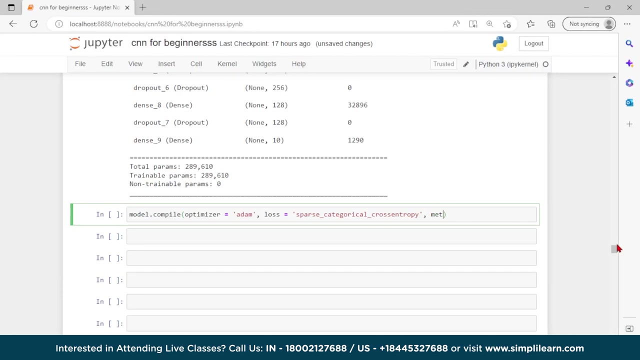 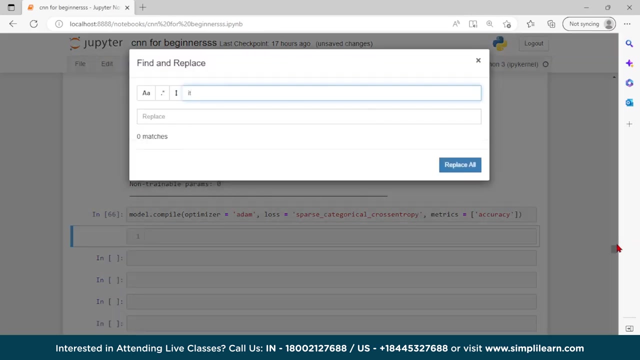 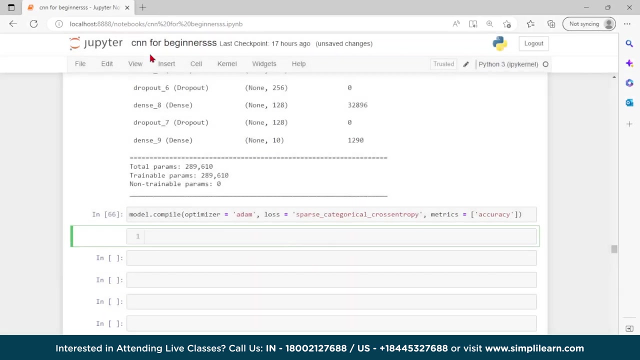 first two small categorical cross entropy: okay, here i will add matrix: first two: accuracy: okay. so now i will write model dot fit: okay, we'll write here- let me delete this model dot fit: extreme train comma: a box first two, 20 batch is first two: five one two comma word post. 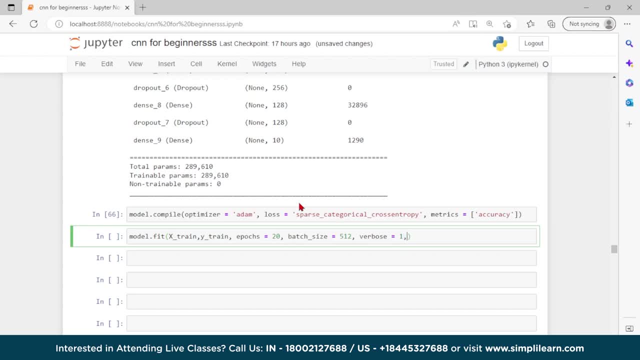 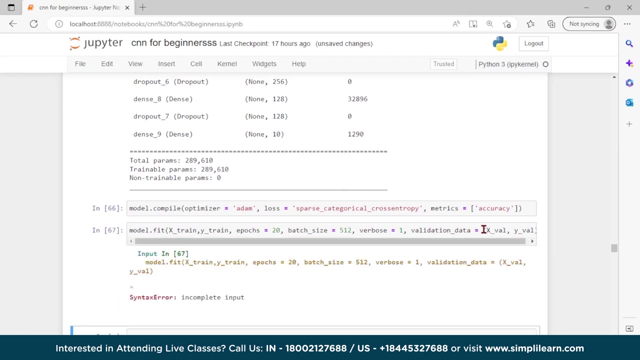 first two one comma. first two five one, two comma. word post: first two one comma. validation data: first two x, where comma y. okay, validation validation data: first two x, Alpha detach and coincide the data. before much zaman now these can just Review right had, If you trying to. 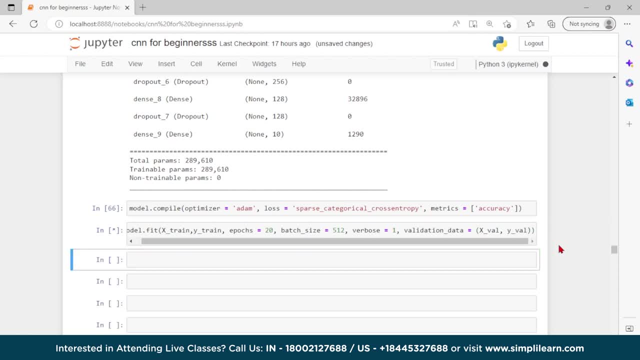 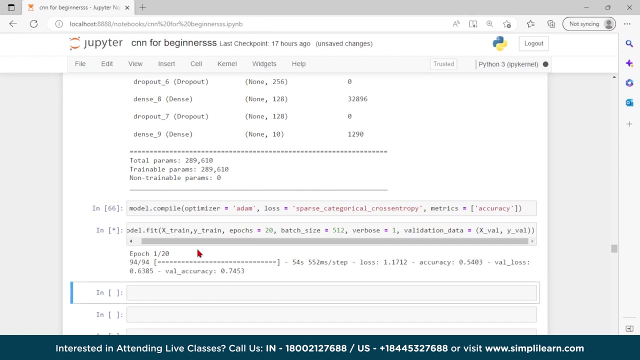 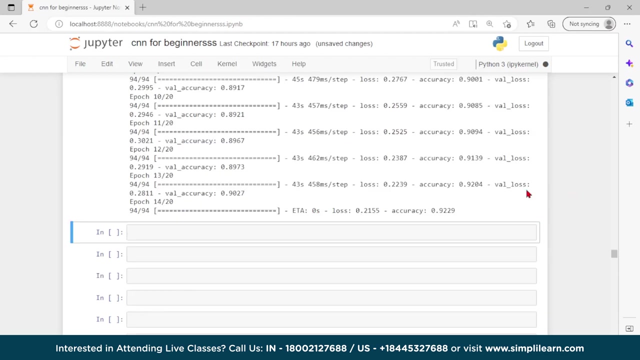 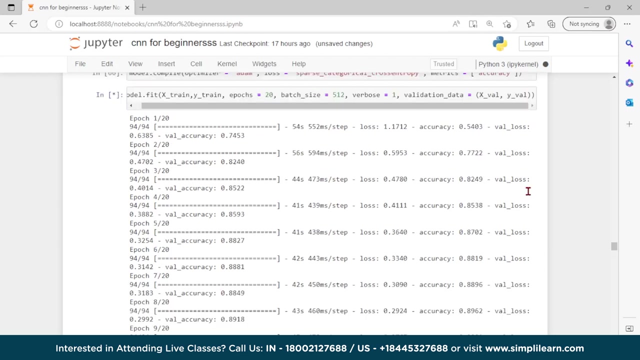 index accuracy. you left h the delivery. uh, this system is the one, the one and come, so we have to wait for some more minutes. they let it be complete. it will hotel 20, so we'll get back to you when it will be complete. almost 14 done: 15, 16, 17, 18, 19, 20 are left. so we'll wait and we'll see. 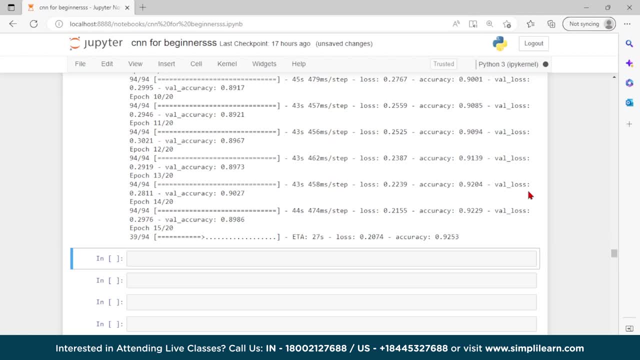 so an epoch is when all the training data is used at once and is defined as a total number of iteration of all the training data in one cycle for the training and machine learning model. so another way to define an epoch is the number of passes a training data set takes around an algorithms. okay, 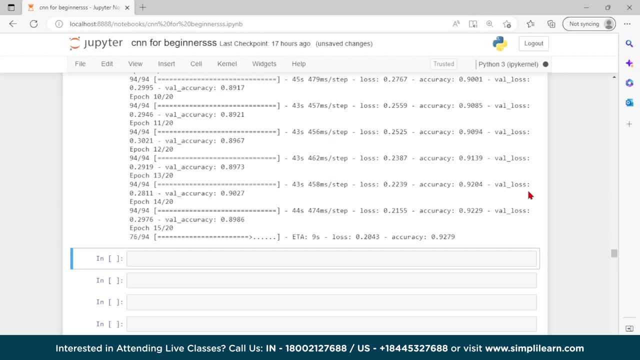 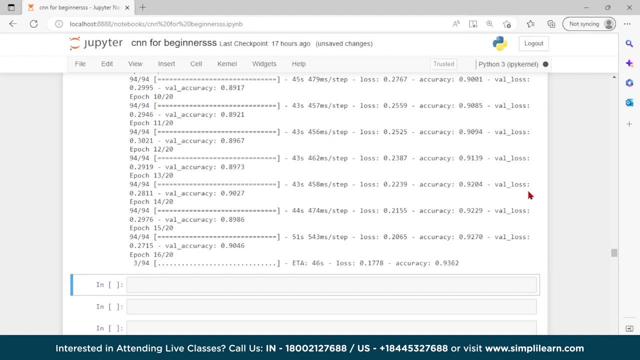 we'll wait till 20, 20, 21, 22, 23, 24, 25, 26, 27, 28, 29, 30, 31, 32, 33, 34, 35. if you want this full code, you can comment and if you have been query related to python. 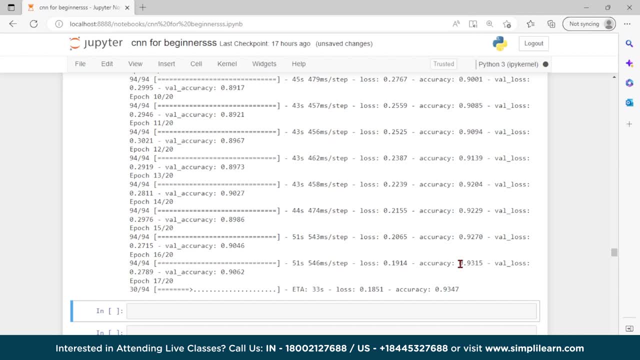 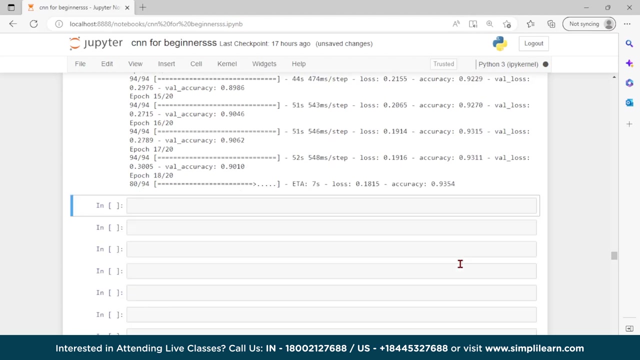 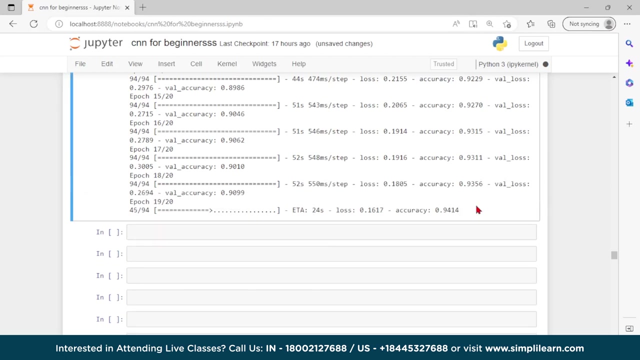 machine learning or anything. okay, you can come on down. our team will reach you as soon as possible. so two more: 19 and 20 ratio. model accuracy is good. 93. you have any query? you can comment down below. okay, 19 is done. final 20s. 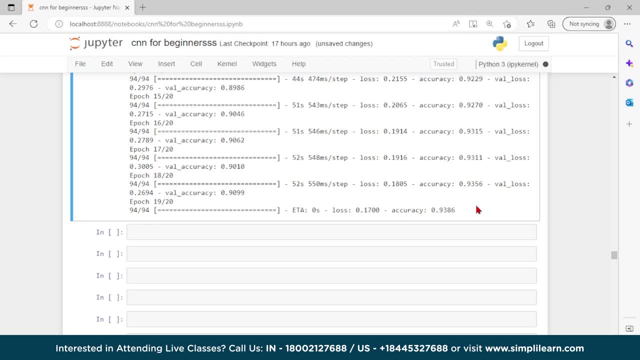 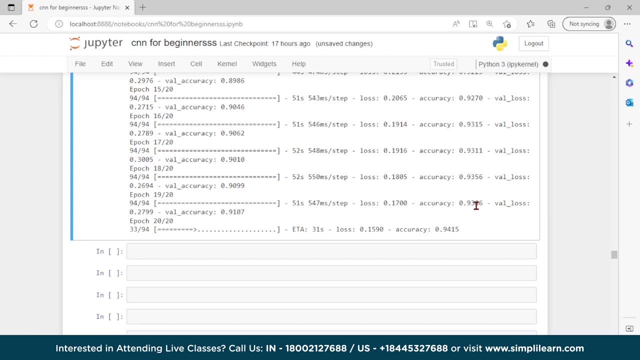 what's going on? epoch, you can enroll in our course of ai and ml. you can check the link in the description box below using course. after this, we will test the model, then we will do evaluation, then confusion matrix and then visualization of the output. the final output. okay, yeah, so it's done. so now let's. 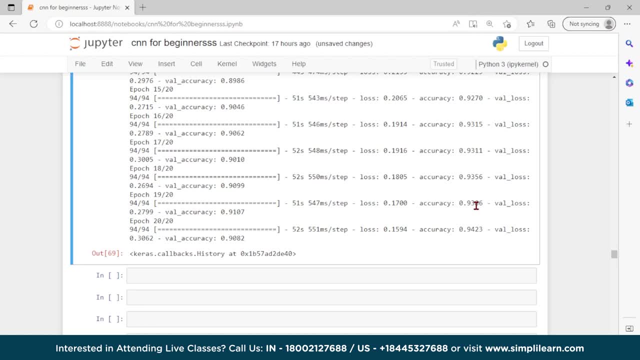 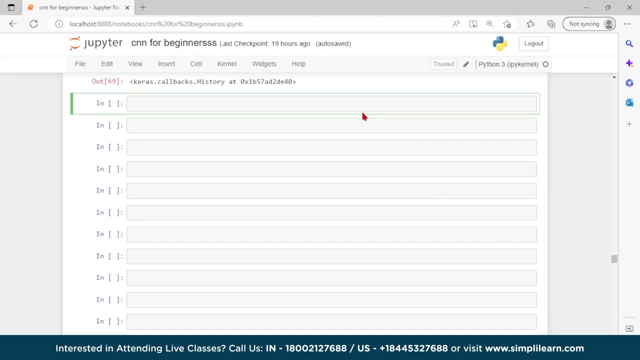 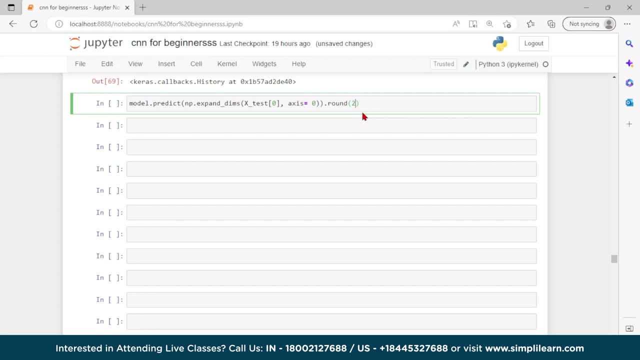 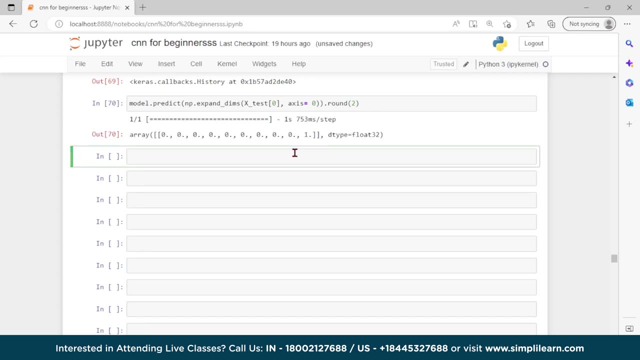 and at zero in zero around zero raised around round is how many decimal points okay. round is how many decimal points okay. round is how many decimal points okay. and model dot predict and p dot expand M's X test. this will be zero. this will be zero. dot round added two. 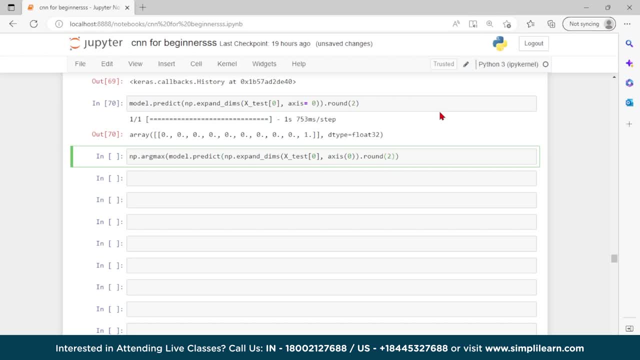 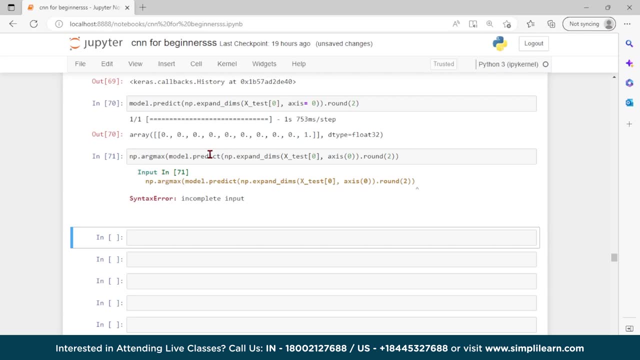 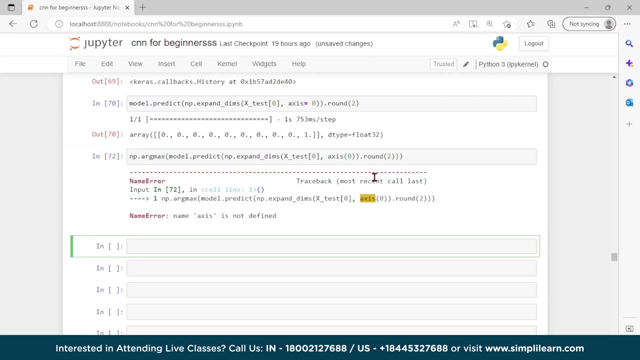 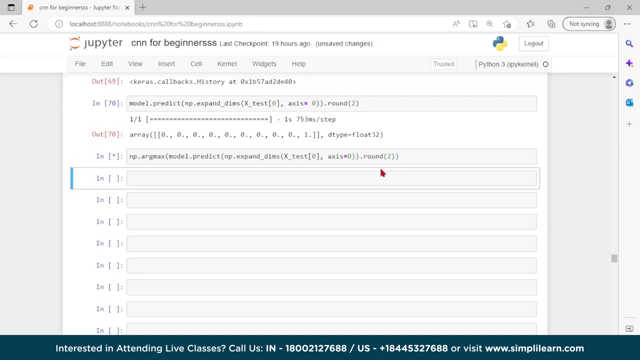 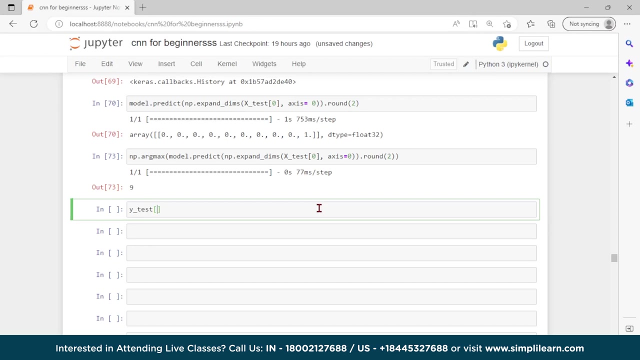 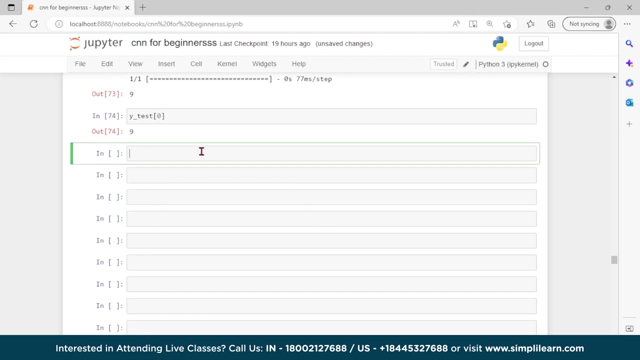 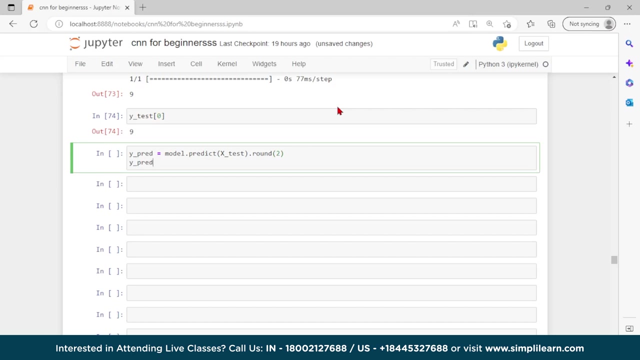 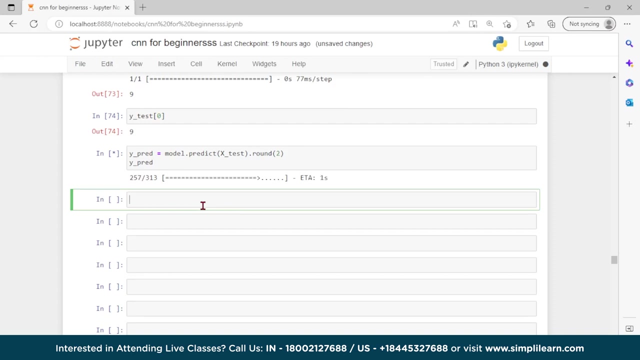 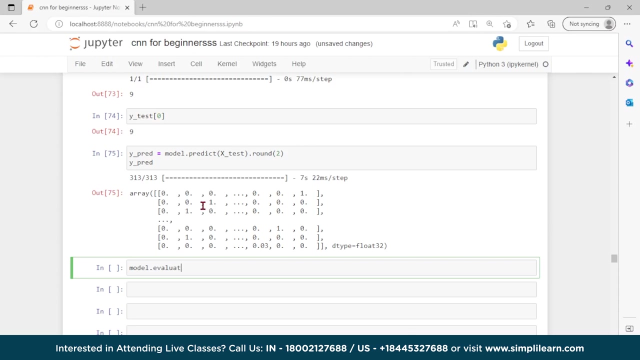 okay, a X is not okay. so here I have to write X equals to zero. okay, so now cross-check my test: zero same. okay. then Y prediction goes to model dot predict and X test two prediction. so now we will evaluate. so model dot evaluate, dot evaluate, test. comma y test. 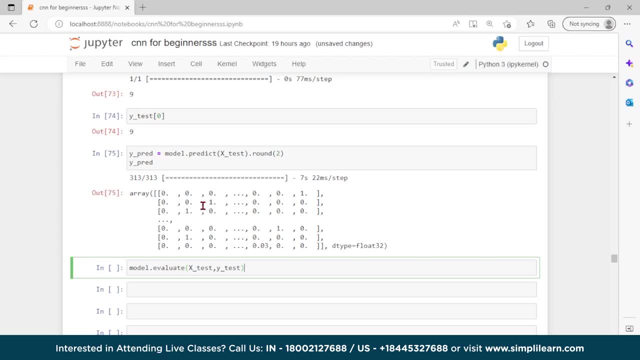 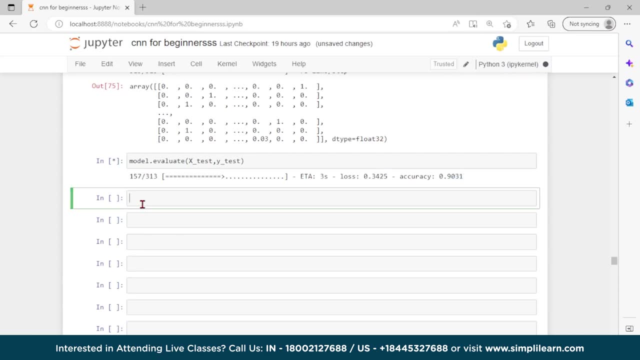 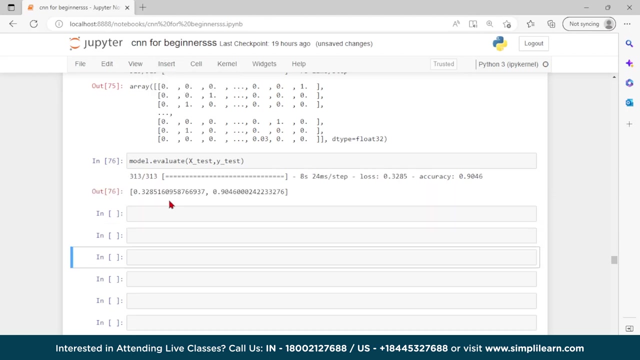 eccentric ventilating. the accuracy given by trend set is 0.94, which is very good, 94%, and accuracy given by test set is 90%. so thus we can say that our model is generalized, so no overlifting or not under fitting. okay, so now confusion matrix. so from sklearn. 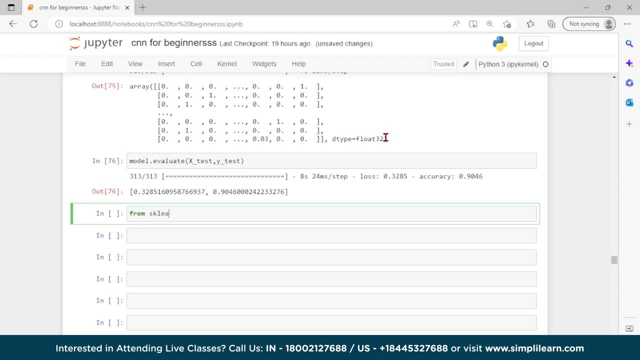 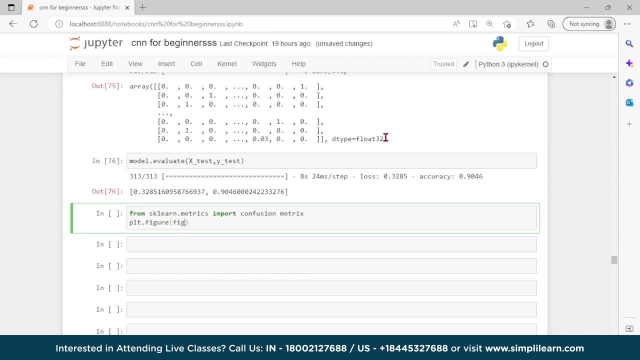 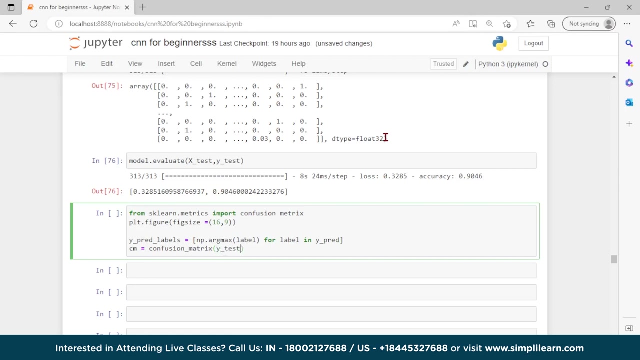 what metrics, both confusion metrics. okay, then PLT dot bigger than figure size, so 16,9 by underscore, prediction by prediction. question np dot arg max 16,9 label or label in by prediction. then cm confusion matrix equals to confusion by matrix, by test by: 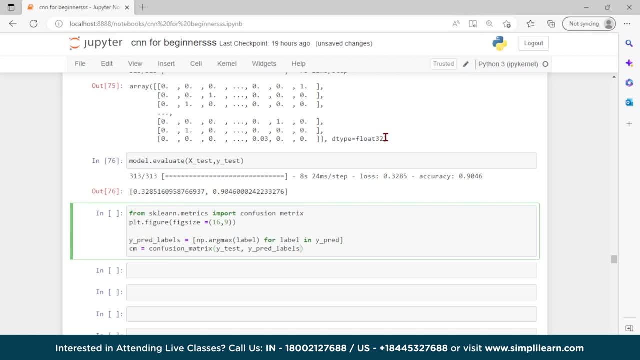 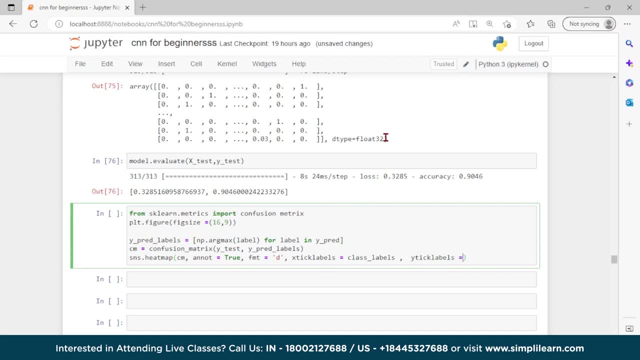 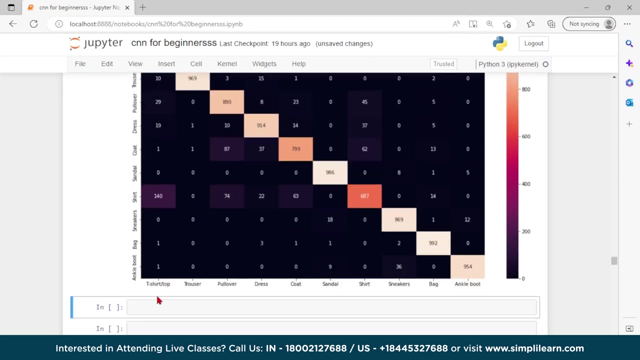 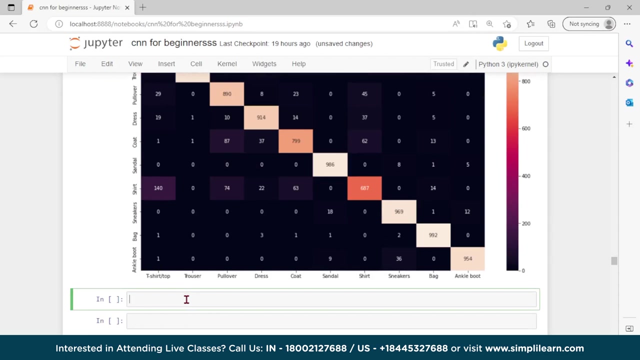 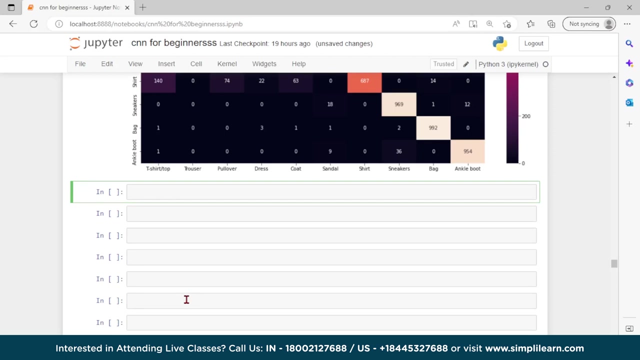 label was to class levels. you, yeah, is another. yeah, see that hit Mavis game. okay, this is for the t-shirt. t-shirt, t-shirt, pullover dress, coat and hair also okay, so now we will visualize the output. so PLT dot. so it is like coming correct or not? 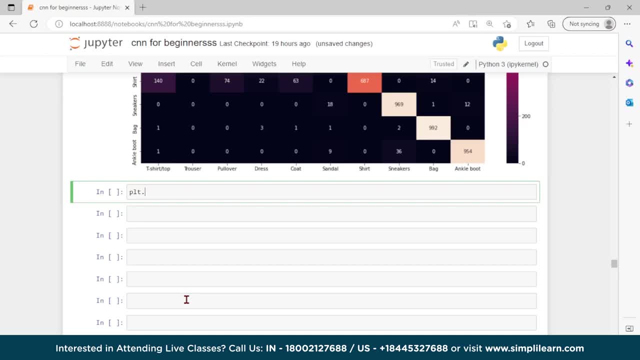 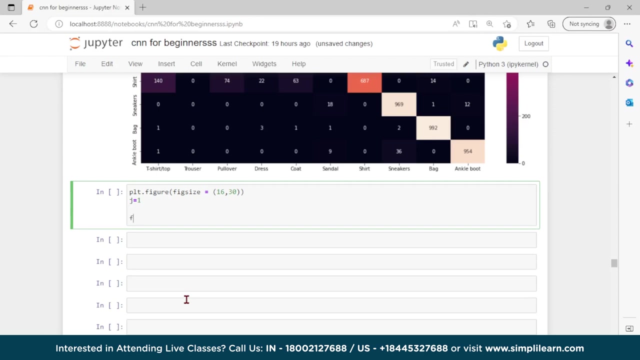 okay, expected and predicted okay. or you can say the actual and predicted. so PLT dot, figure, you, you, you, you, you, you, you. the size: the size was to 16, comma 30, a equals to 1, or I in NP, dot and um, no and int. 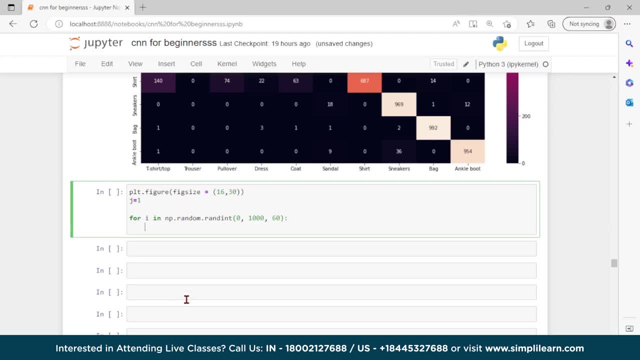 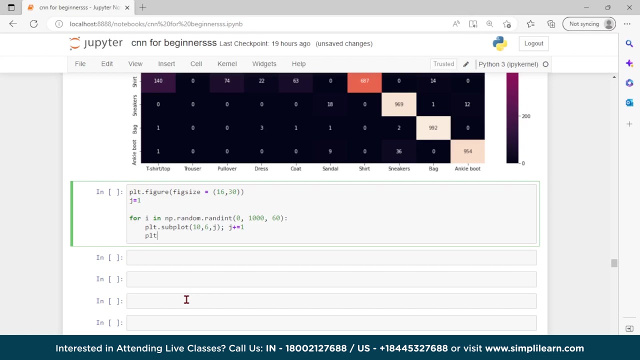 60 reality taught subplot x. come on. yeah, then here I will add J plus 1 plus 1 and PLT dot. I am sure X test I shape date. it's 28 height and width and see map equals to grace here t dot excess of. 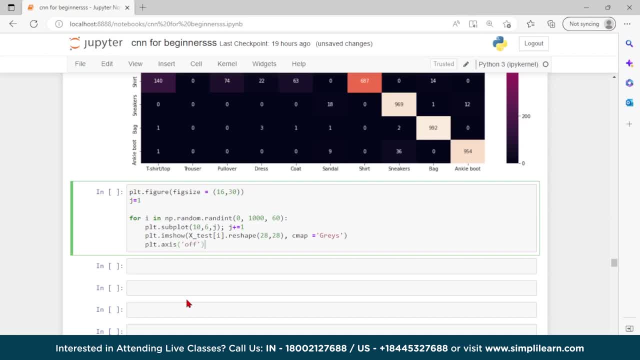 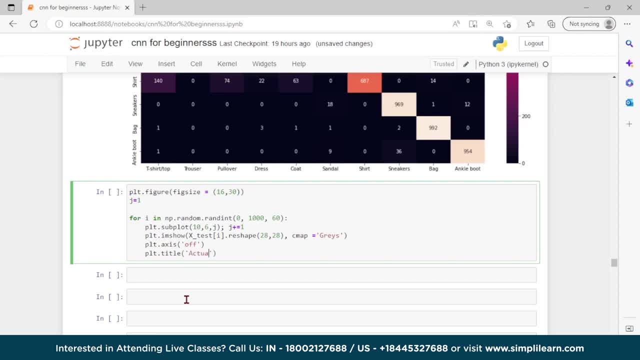 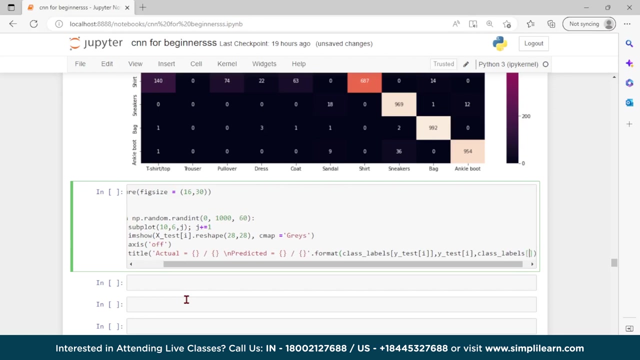 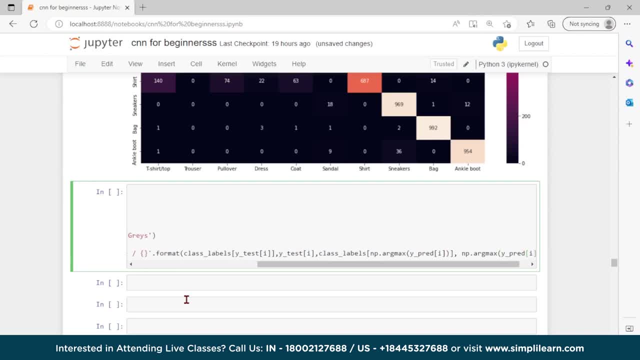 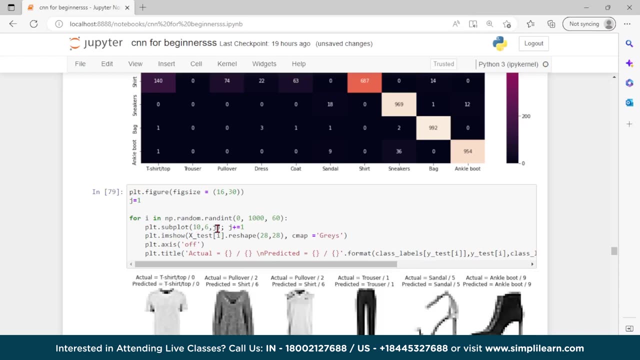 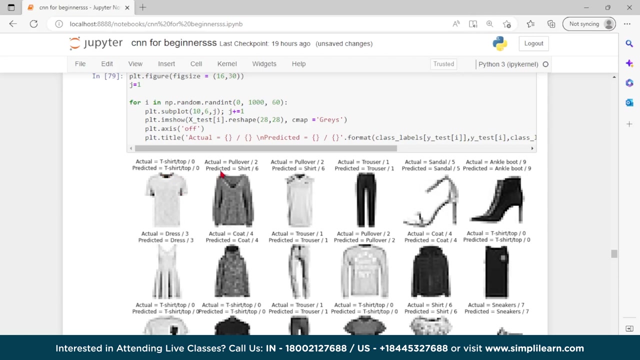 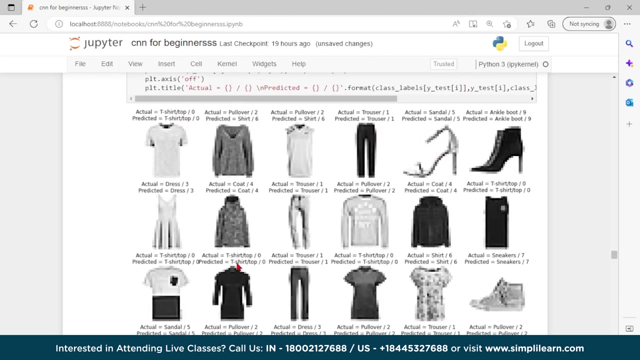 nb dot, nb, dot, nb, dot. predicted. i press enter loading. so as you can see, actual is t-shirt, shop t-shirt and top. then predicted also fine, ok, some error. then trousers are same, sandals are same and then ankle boots also same. so, as you can see here, 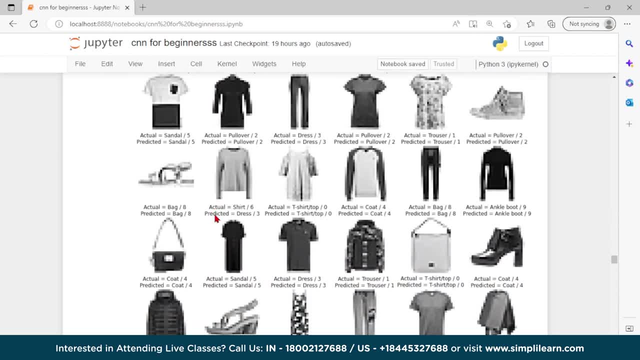 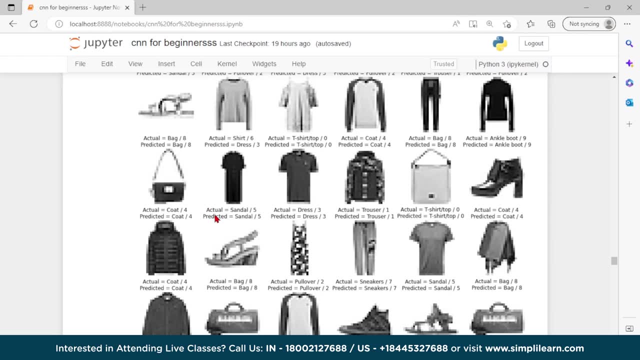 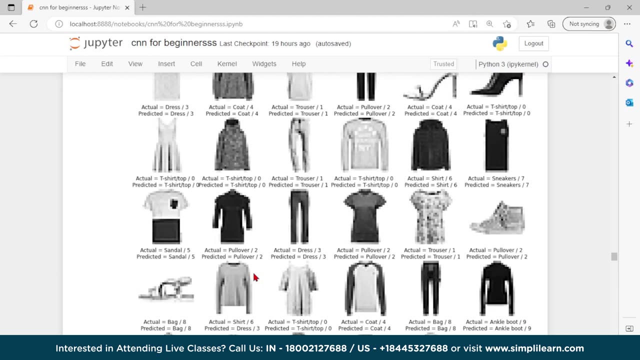 some are right and some are wrong. see, because the testing accuracy is 90%, the predictive accuracy, that the training accuracy is 94%. that is why, ok, so this is the CNN of image classification, how you can use and, if you have any queries related, any code.